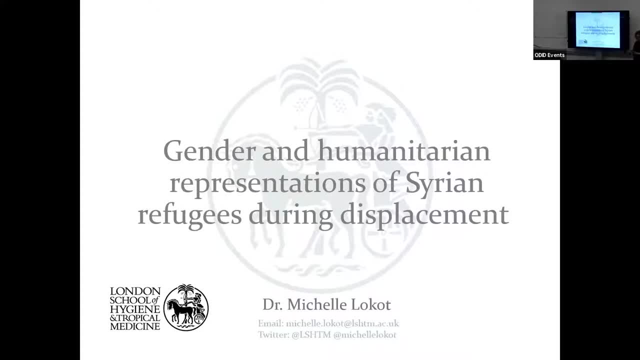 Michelle takes an interdisciplinary approach to conducting her research. Her research interests abroad, considering forced migration. She's engaged in gender humanitarian assistance and research methods, And she's experienced in conducting feminist research using participatory approaches. Two recent publications of hers that might be of interest to you are in frontiers of sociology and refugee survey quarterly. 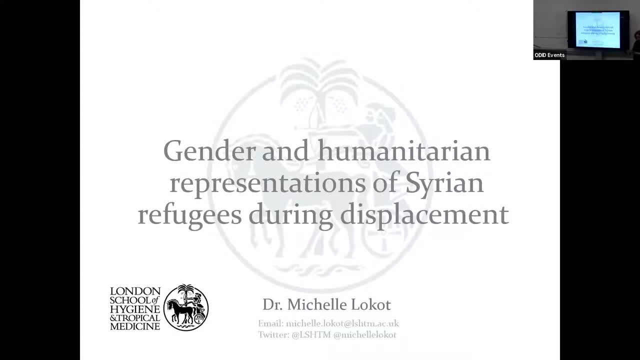 and they focus on gender mainstreaming and organisational culture and aid sector and humanitarian accountability. The title of our talk this evening is Gender Equality and Representation of Syrian Refugees during the Second World War. Michelle has kindly agreed to talk for around 30 minutes and then take any questions that you might have. 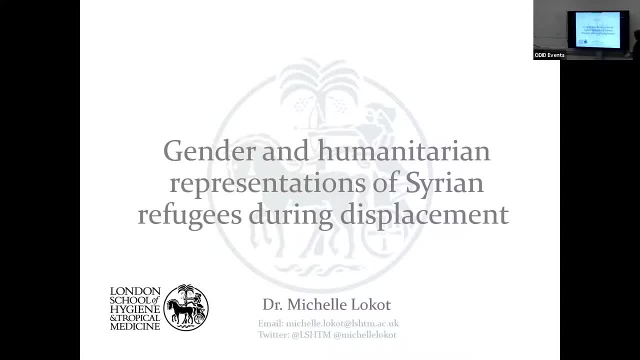 So please do use this opportunity to ask her about her presentation today, about how her publications work for you- And potentially I know that some of you may also be interested in feminist research methods as well- and how they can be applied in practice. 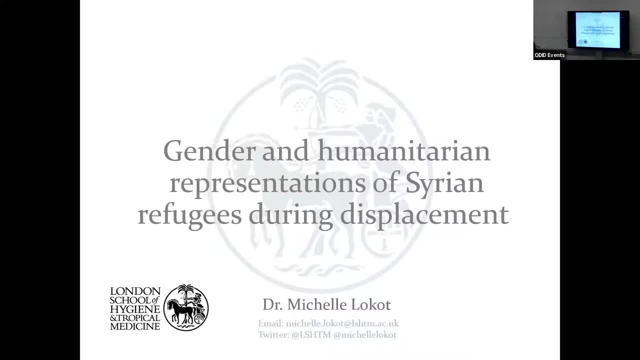 Thank you very much. Thanks, Catherine. It's great to be here today and speaking on. Today. I'm going to be speaking about gender equality, Gender equality changes during displacement And focusing on this narrative that gender non-change is something that happens during displacement. 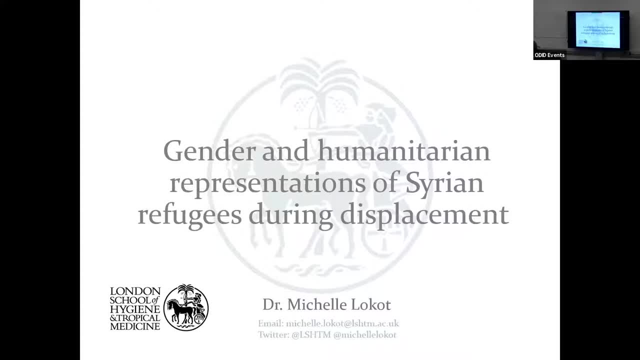 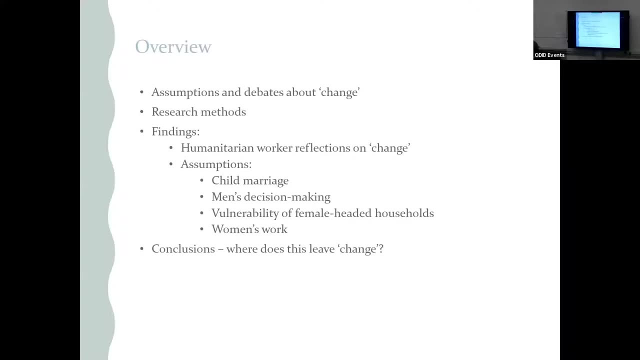 and displacement is an external intervening stressor that causes change among refugee populations. So I'll start off just by situating what I'm speaking about in some assumptions and debates about change during displacement, And then I'll talk through my methods, which Catherine mentioned include feminist research methods. 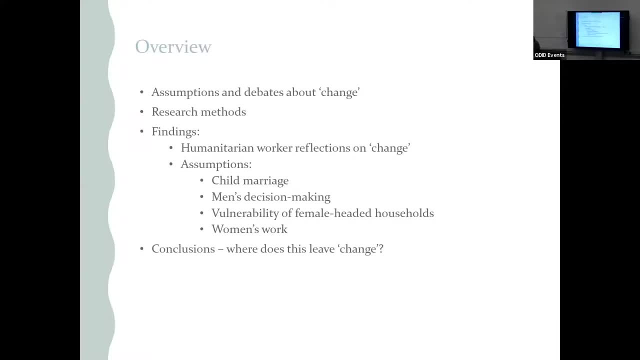 and then perhaps my findings, And I'll start off by sharing the findings and reflections from humanitarian workers on this concept of change. What does it mean? What does it look like? Who defines change? And then I'll focus on four assumptions that are often made about change among female refugees. 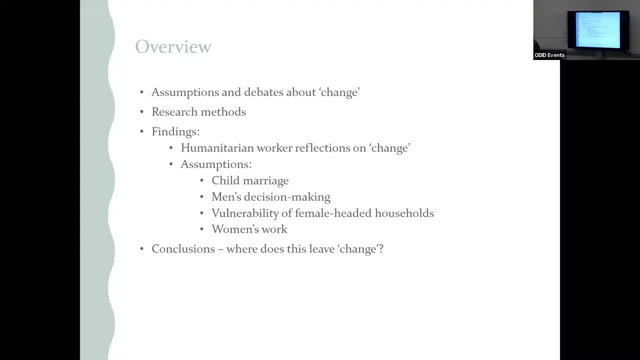 The first is around child marriage, The second is around men's decision making, The third is around the vulnerability of female-headed households And the last is about women's work. I'm going to give some general reflections on what it might mean for scholars. 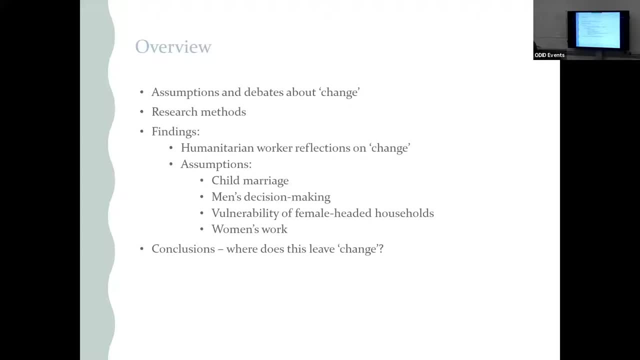 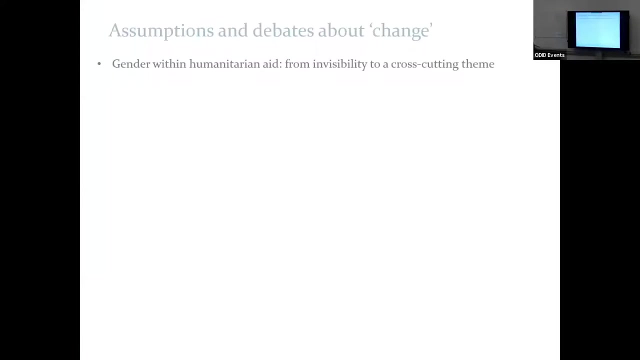 What it might mean for practitioners to conceptualize change during displacement. And today I'm speaking on my PhD research, which was among the self-written series of the book. I'm starting off and trying to sort of think about some of the assumptions and the debates that informed this research. 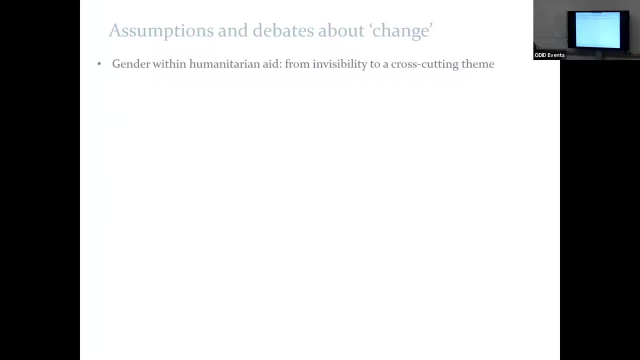 And really I think an important starting point is thinking about the narratives about gender and displacement within the history, of how gender has been placed within humanity. So humanitarian actors were historically critiqued for rendering women invisible in their humanitarian activities, And so gender analysis became a way to rectify this. 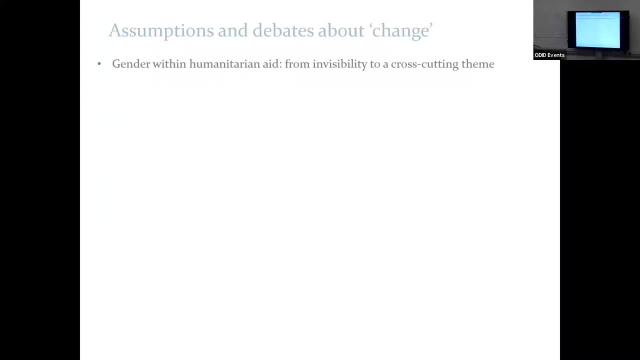 Since the 1990s there's been considerable progress that's been made in trying to bring women into sort of development and aid agendas. Initially it started with sort of approaches around gender balance and trying to make sure that women were also recipients of aid. 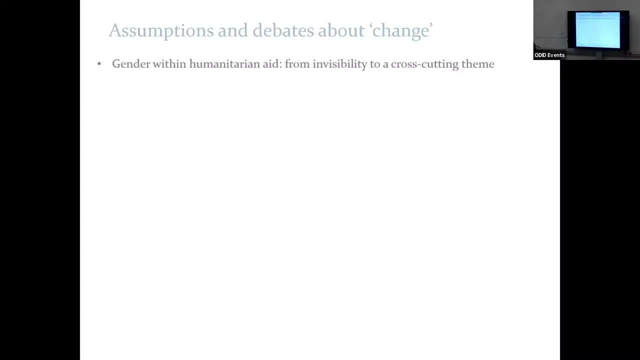 And then, in recent years, it's become more and more common. It's included a focus to considering hierarchies of power surrounding women's lives, So now gender equality is increasingly mainstreamed in humanitarian action. Gender is seen as a cross-cutting theme to be addressed across all sectoral programs, as well as an issue in its own right. 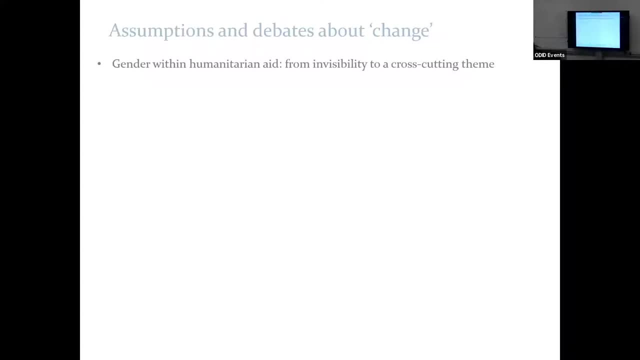 And gender analysis is often a donor requirement, particularly for new programs. Through gender analysis, we can see narratives about displaced populations becoming institutionalized, And so my particular interest is in how gender analysis about refugees is presented and what kinds of dominant narratives might inform this analysis. 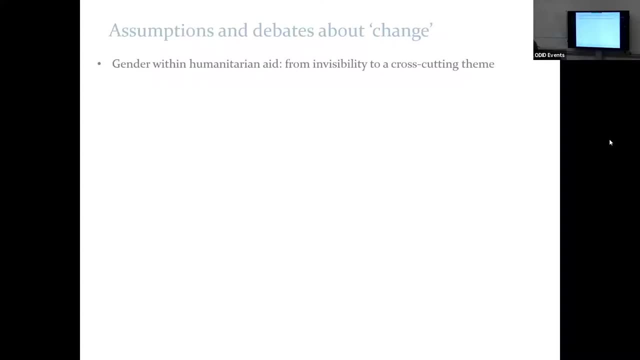 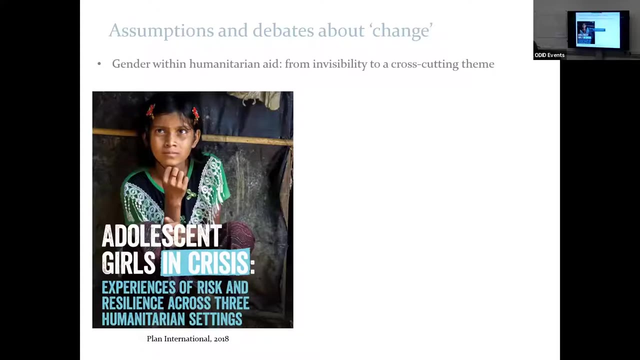 So I'm aware the term refugee is not neutral, but it's political and it's also gender. So, for example, there's often a focus on the female refugees as vulnerable, as powerless, But we see quite a different narrative about male refugees. 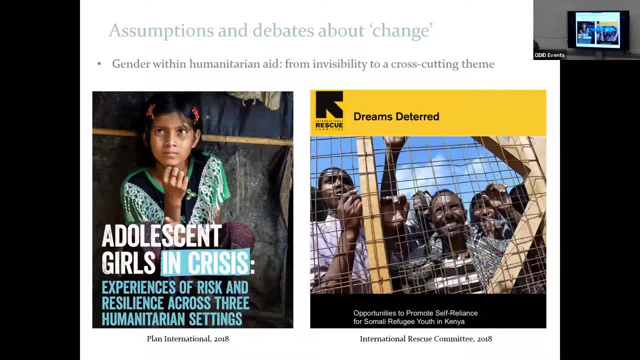 Media and news outlets in particular are looking to male refugees as vulnerable And dangerous in how they move across borders, And there is a very political way that gender can be changed: the way that refugees are spoken about. The term refugee is also sometimes used as a way to reflect on a collective refugee experience, which you may explore if you have the opportunity. 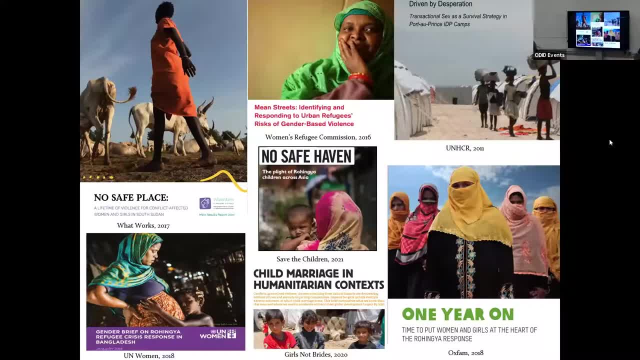 And there are very particular narratives that emerge around gender and displacement. So displacement is positioned as an expression of a gender identity And it's a very important narrative. So displacement is positioned as an external intervening force that results in very particular changes And, according to humanitarian action, these changes are really similar across different settings, different types of conflicts. 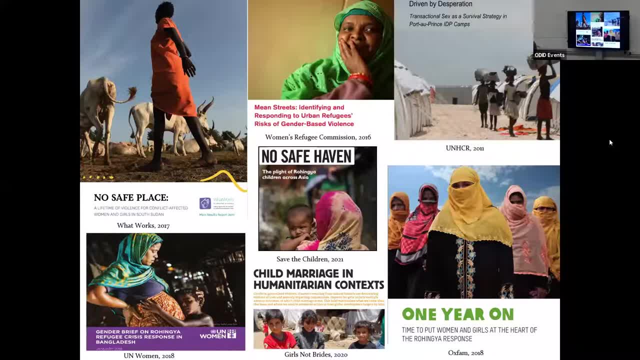 And they often focus solely on women's experiences, So they often include things like soaring gender-based violence, increased child marriage, increased economic pressure on women, sexual exploitation experienced by women and girls, and broken and disrupted family structures. And in these narratives, culture and tradition are often positioned by humanitarian actors as negative forces that result in narrow-minded decision-making among refugee populations. 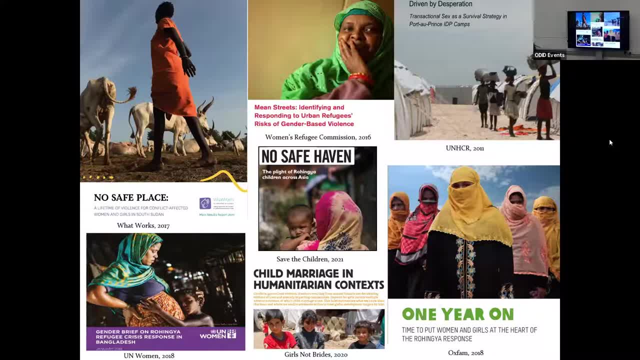 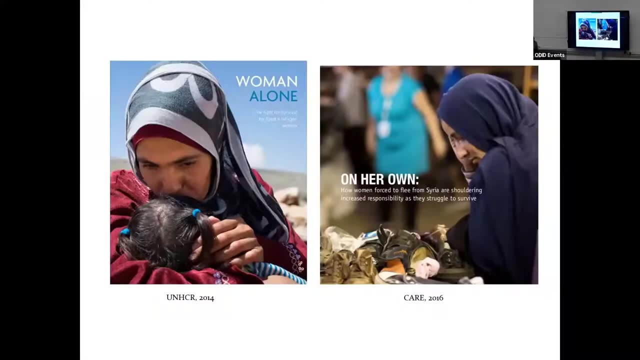 And that result in refugees resorting to harmful practices as a coping mechanism, And so examples of such analysis are also present in reports about Syria. specifically, A very dominant narrative is that families have been torn apart, That women are heading households for the first time, 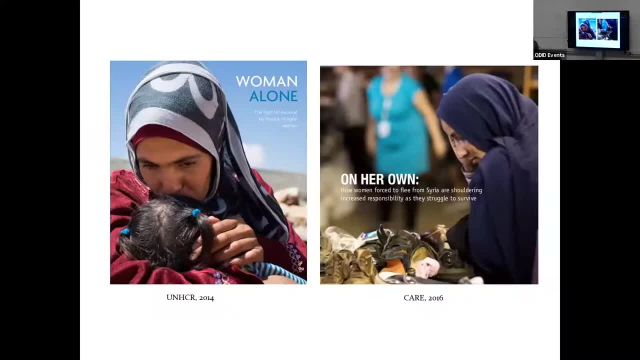 While men have passed away or are out of the way of fighting, And Syrian refugees' lives are thus depicted as shaped by disruptions to social structures and systems, by impunity and lack of law and order. Multiple reports state that men cannot work and therefore they feel they're not fulfilling their traditional norms. 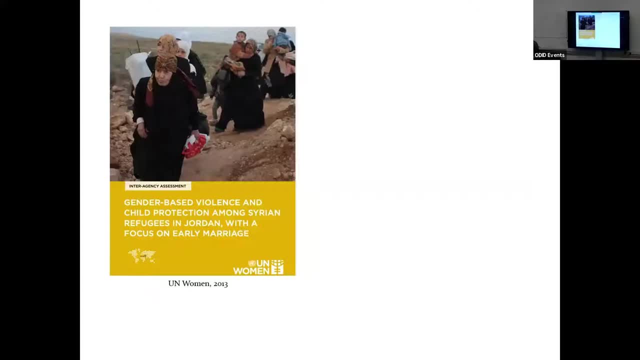 And this leads to them using violence against women. In reports issued by humanitarian actors, gender norms are always described as patriarchal, But often without clarification on what these norms were like before displacement. Gender-based violence and gender norms in general appear almost in a vacuum. 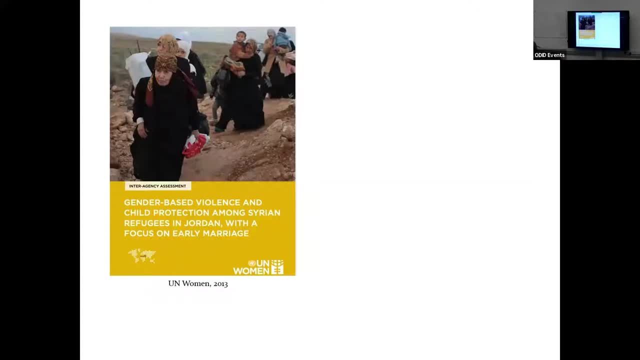 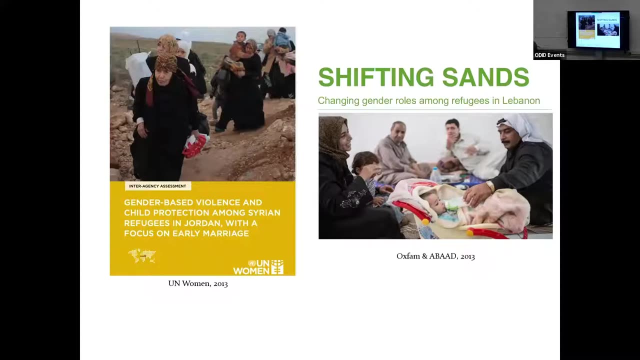 As if these were non-existent prior to war. Some agencies acknowledge that changes in gender roles are complex And that there are stronger claims about gender roles being reversed. For example, women are described as engaging in economic work during displacement, apparently for the first time. 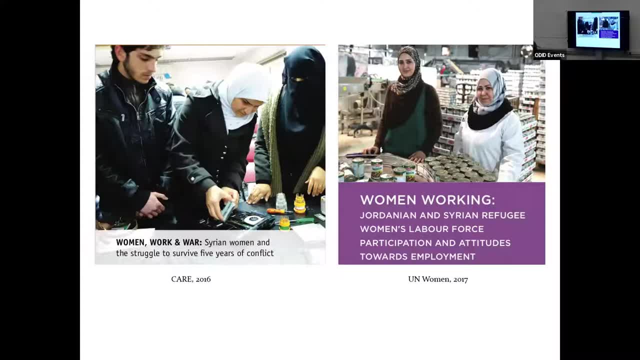 While the narrative is that men were the sole economic providers prior to war, In these narratives refugees are disempowered and halted. But their shift to being empowered is through being trained, having their awareness raised, accessing assets and opportunities through humanitarian actions. 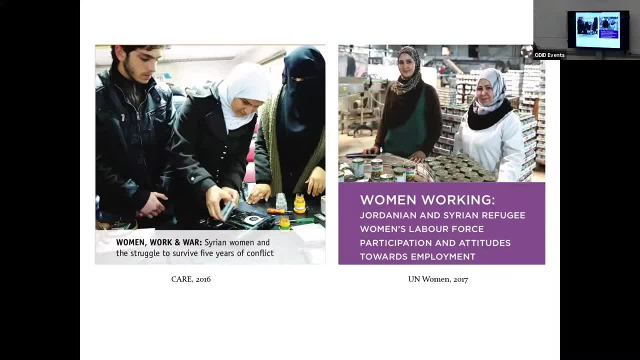 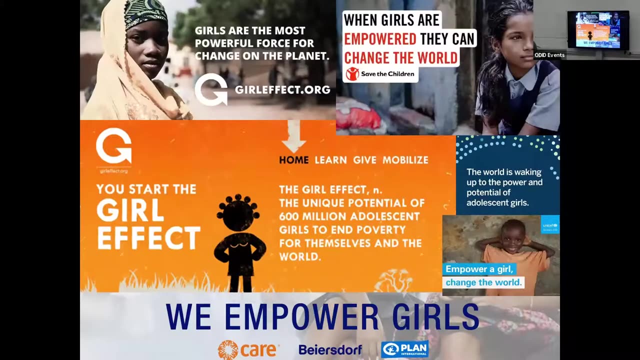 And this is part of the pervasive and also the quite powerful narrative about the empowerment of women and girls. This is a neoliberal narrative that at times instrumentalises these girls Not placed as a solution to poverty. So an example of this is the popular Girl Effect YouTube video. 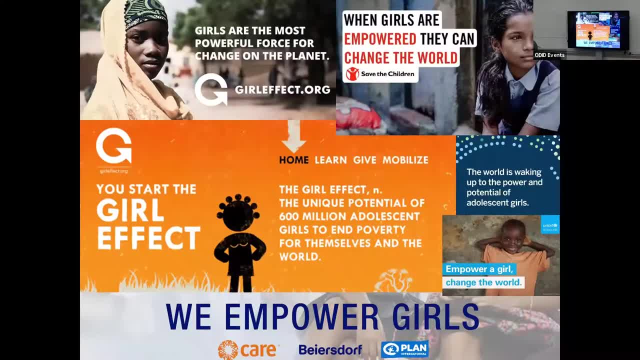 And this declares girls to be the unexpected solution to poverty, age hunger and war. The message of the video is: invest in a girl and she will do the rest. So, during displacement, it's really interesting to see that this narrative takes a very specific trajectory. 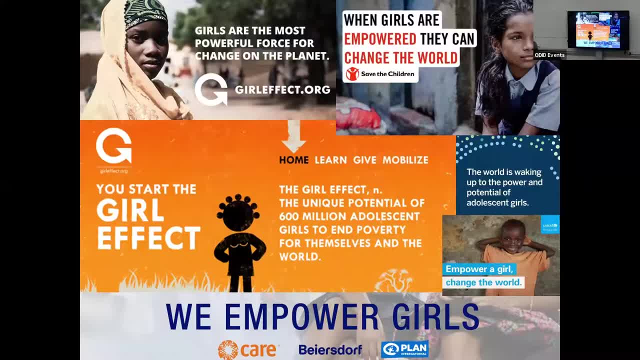 Refugees, and refugee women in particular, are disempowered by default And they need to be empowered by humanitarian actions So that they can develop skills, so that they can know their rights, so they can protect themselves And then, ultimately, so that they can become productive actors. 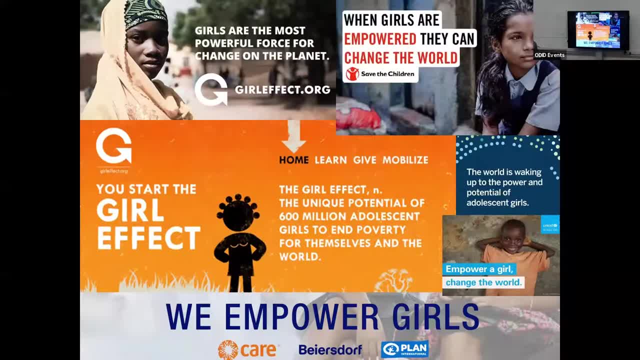 The idea of a female household head carrying the burden of her family upon her shoulders is part of the empowerment narrative, And these narratives have been critiqued by scholars and activists, including those who seek to decolonise humanitarian aid. So my research is really situated within these humanitarian narratives. 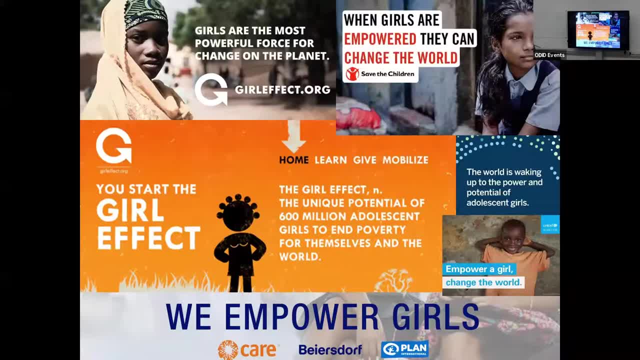 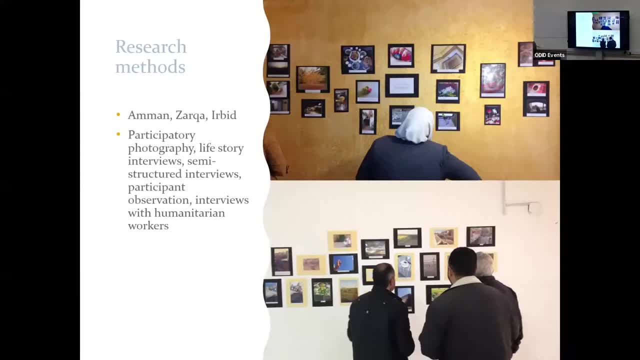 And it's also in focus on my own experience working and being entangled in some of these narratives around gender equality and women's empowerment. The research that I conducted was conducted over nine months of fieldwork in 2016 to 2017.. And I interviewed Sarah Murray in the 1860s, who lived in the Jordan cities of Hamas, Obeid and Saqqa. 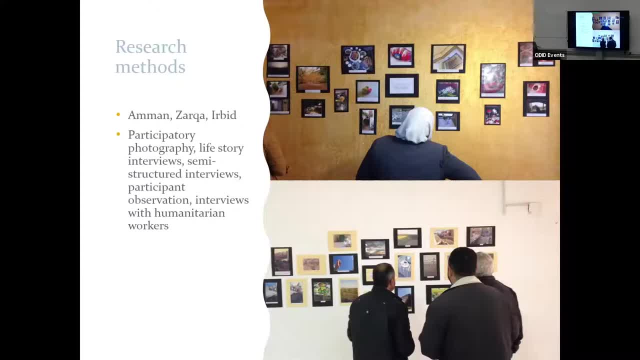 My fieldwork began with participatory photography workshops, where refugees had the opportunity to discuss their day-to-day experiences using photography, And, within these workshops, I held focus group sessions where refugees talked about gender roles and they talked about their day-to-day experiences both in Jordan as well as in Syria. 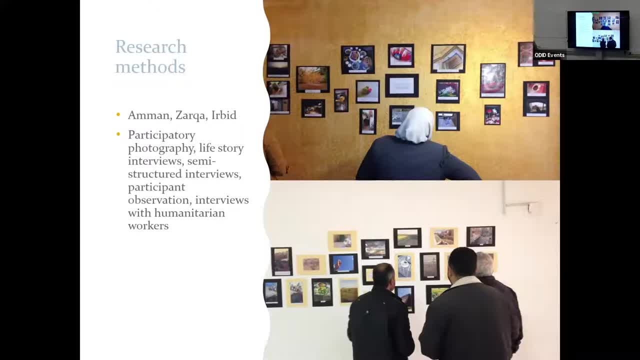 Participants from workshops were invited to join semi-structured interviews or participate in multiple longer backstory interviews, And these took place in capital, In parks and people's homes across the cities, And it's one of those that also conducted interviews with international and national humanitarian workers. 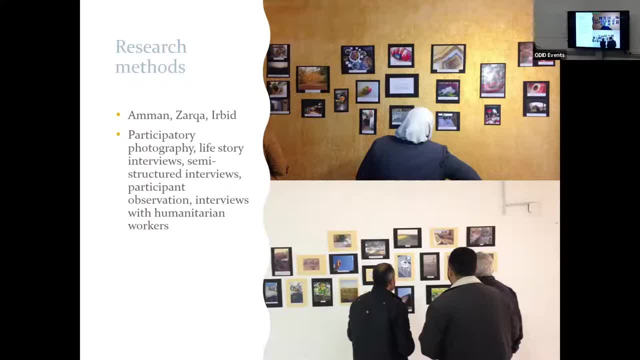 And some of those I'll reflect on a little bit today. So my research is informed by a feminist perspective which seeks to sort of counter this often extractive, sometimes top-down approach to research that humanitarian agencies sometimes undertake when they're engaging with refugee populations. 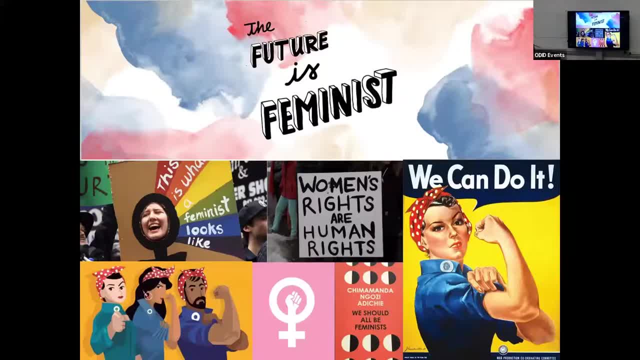 So one is feminism. Feminist research looks to improve women's lives and to seek, at least to try to unravel and address and challenge the power hierarchies that structure their lives. It recognises that women's lives are multiple, intersecting power hierarchies and identities. 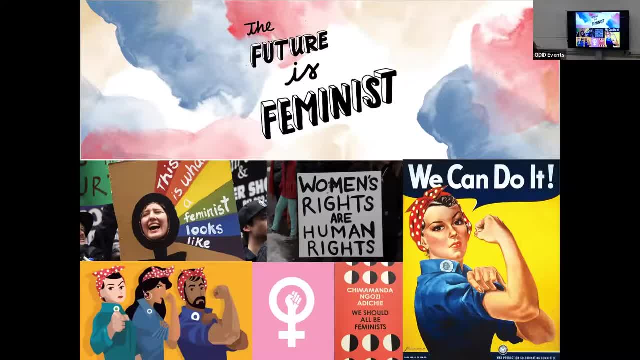 And it's really looking to take an intersectional approach to actually understanding women's lived experiences, Recognising there's not just a homogenous women's life, Not just a homogenous women's experience, But that things like race, age and socioeconomic status can be really powerful factors that intersect with gender and affect their lives. 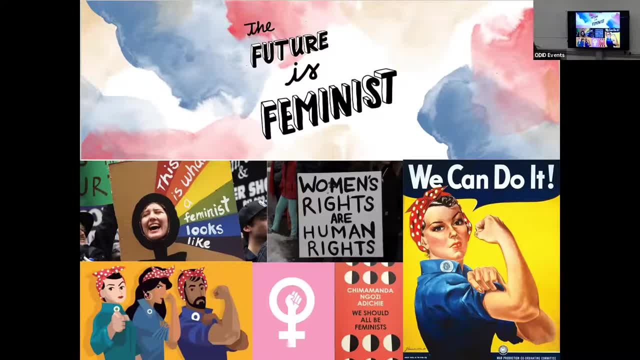 And so Feminist Research Takanoa also recognises the way that humanitarian structures can reinforce new colonial power dynamics, Creating a culture of white saviour whose task is to rescue Middle Eastern women from being forced into harmful practices. So Chakrabarty's feedback talks a little bit about saving brown women from brown men. 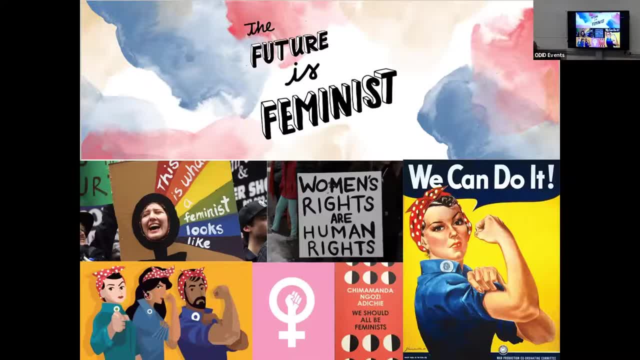 And I think this is really relevant here when thinking about the role of humanitarian actors in implementing activities that seek to promote gender equality and women's empowerment. And so, for my research, following a feminist approach meant really trying to unravel the power dynamics between myself as a researcher and my research participants. 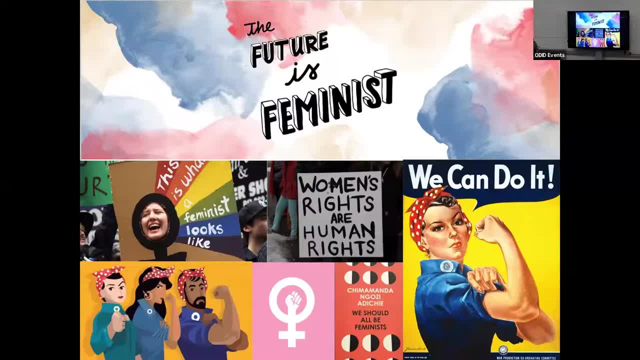 And so this is about not just about the methods themselves, But the way that they're implemented. So for me, it meant not just using participatory methods or more participatory methods like photography and focus group discussion, But also implementing the research really intentionally in a way that would seek to challenge the traditional ways that we do research. 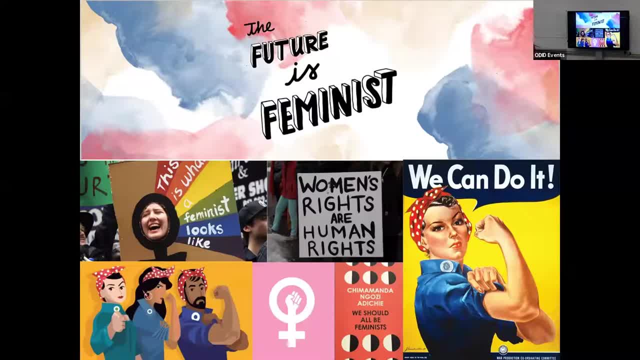 So, for example, this meant for me allowing refugees to speak about issues that they wanted to speak about, Instead of sort of being rigidly stuck to my interview guide, And for me this resulted in lots of change. There were lots of tangents and exploration of issues that I didn't originally plan to take them in at all. 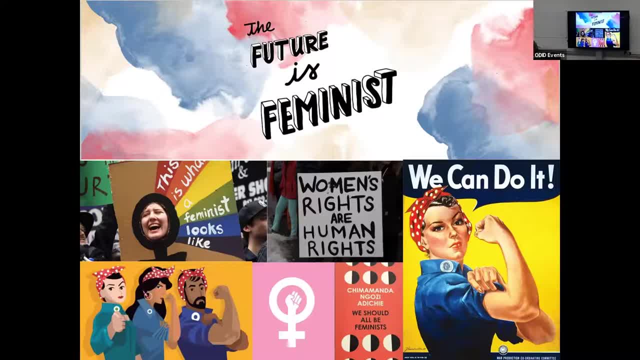 It also meant engaging in reciprocity, So helping refugees to find information about humanitarian services, Helping to connect them or follow up on cases where they weren't sure that they were entitled to or were waiting to hear back from different UN and NGOs. It also meant spending time socializing. 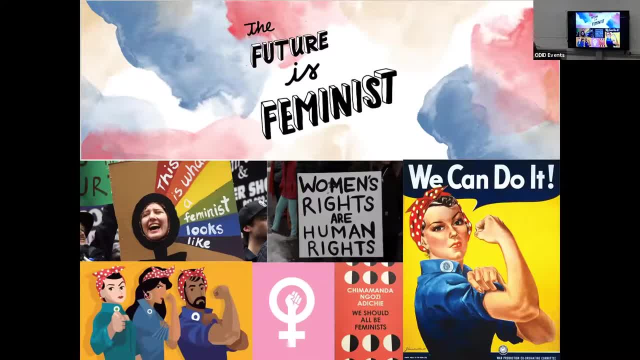 Instead of taking an extractive approach to collecting data. So I spent a lot of time Drinking lots and lots of coffee And eating all kinds of delicious food, Learning how to cook different food And part of that process of getting to know people over that nine month period. 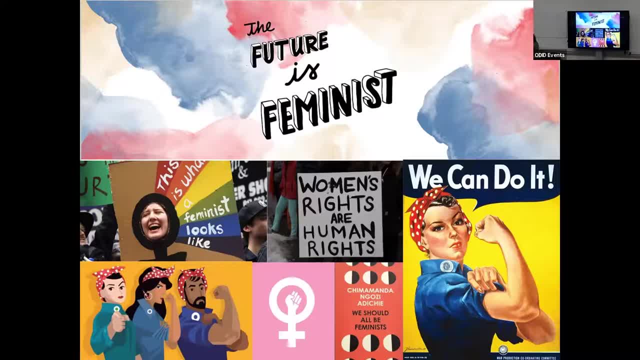 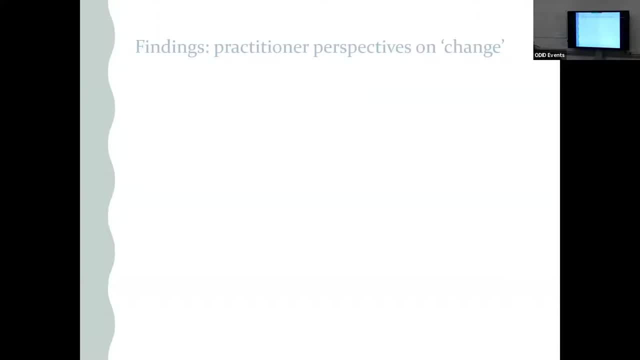 Okay, so, moving on to the final group, I'll start off with just a few reflections from humanitarian practitioners about gender norm change, And then I'll talk about the four areas where assumptions might often be made about gender norm change. So practitioners often discuss the gender issues faced in terror refugees as if these were a given. 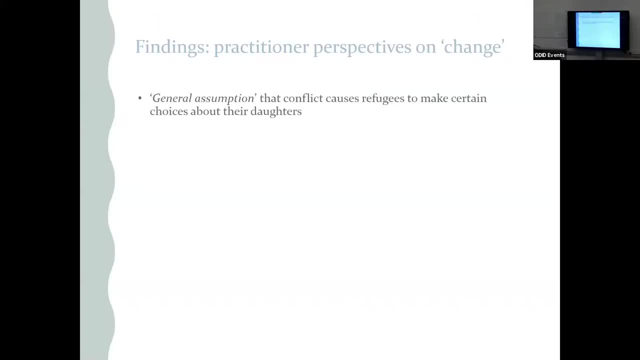 One participant reflected on what she termed this general assumption to assume that, because of conflict, refugees would automatically make certain choices about their daughters. There was this idea. she felt that refugees behave in particular predictable ways during conflict And that their actions inevitably cause harm to girls. 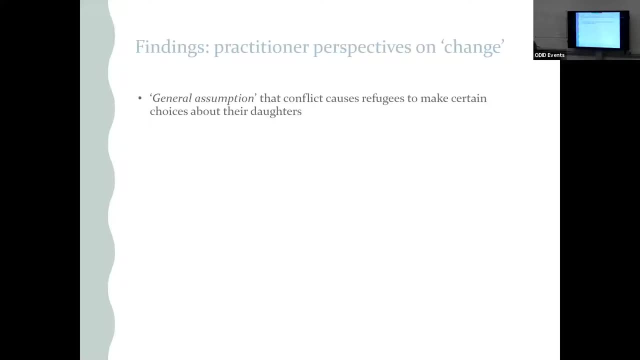 Another practitioner discussed how refugees were treated, in particular, predictable ways, during conflict And that their actions inevitably cause harm to girls. Another practitioner discussed how the mobilisation to respond to child marriage meant the social importance of marriage And she said, on some of the issues like of early marriage, the initial kind of worldwide, you know, cry against the Syrian girls was really, was really harmful. 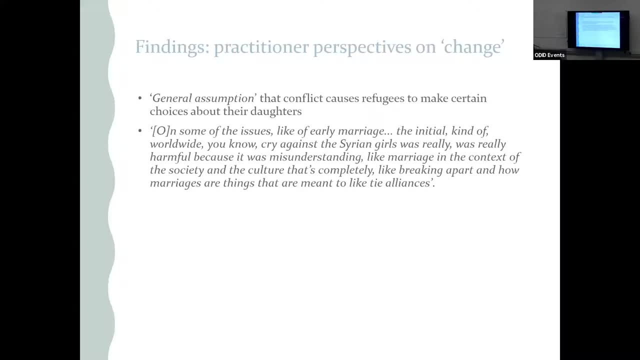 Because it was misunderstanding marriage in the context of the society and the culture. It's completely like breaking a heart And how? marriages are things that are meant to tie alliances, And so, for this practitioner, the visibility of child marriage Resulted in the practice being framed very negatively by humanitarian actors. 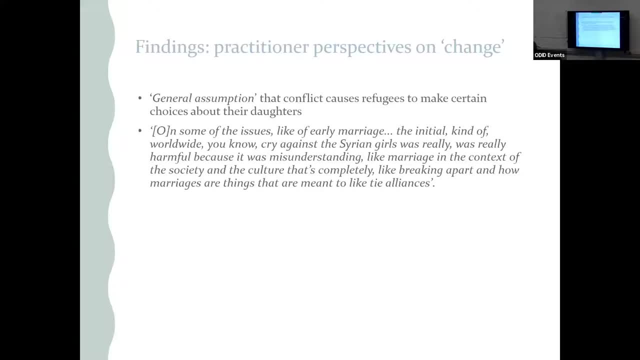 Instead of being understood and presented as a practice that was designed to bring families together. Humanitarian actors also talked about the changes they sought to achieve through their activities- Changes in gender norms- And, as part of this, they discussed the pressure to demonstrate that their actions and their programmes could, in fact, bring about change. 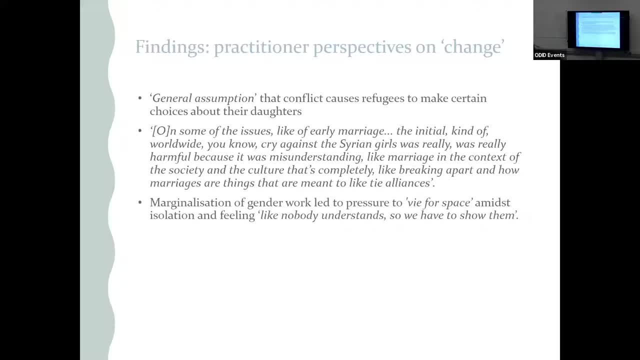 So one consultant said that the marginalisation of gender and gender-based families, Programming within the broader humanitarian sector, Led to this constant need for staff while working on these issues, to vie for space. This reinforced the culture where staff felt isolated, Like nobody understands. so we have to show them. 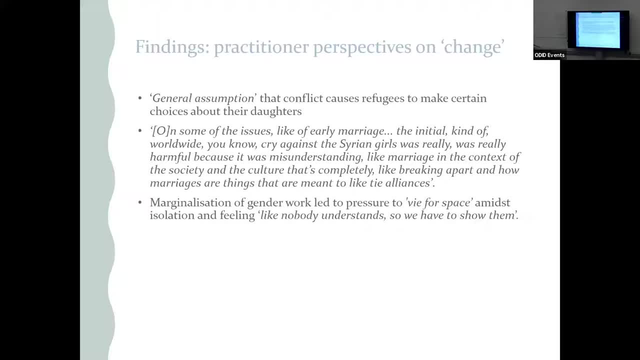 So, for example, she felt pressured to express confidence that their programme would result in gender-based violence by armed men ending And having to make those kinds of promises and determinations. Measuring change was also discussed by practitioners as being particularly challenging. One practitioner talked about measuring change in gender-based families and child marriage. 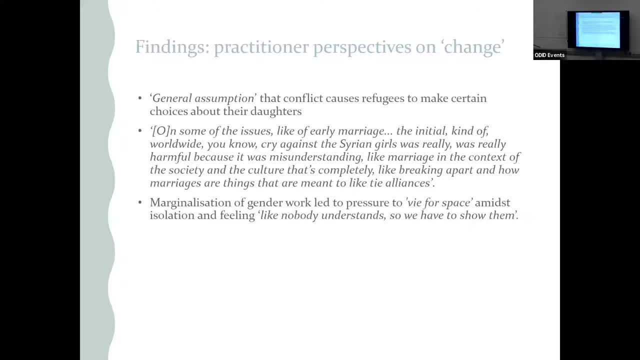 And observed it's extremely difficult to show results. Want to know what indicators will you use to measure that? Another practitioner noted. how are you going to measure it? It's so hard. For one humanitarian consultant, the issue was capturing complexities in changes across diverse locations. 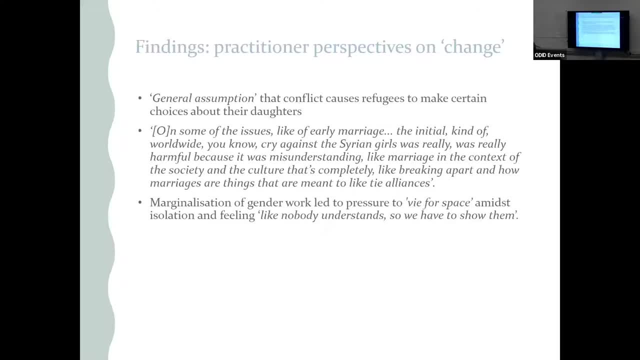 She commented, change looks different in different places, And so, with this really brief overview of what practitioners found and how they positioned change, I want to focus the rest of the time looking at these four common narratives about Syrian refugee populations And really drawing on the ethnographic data that I collected. 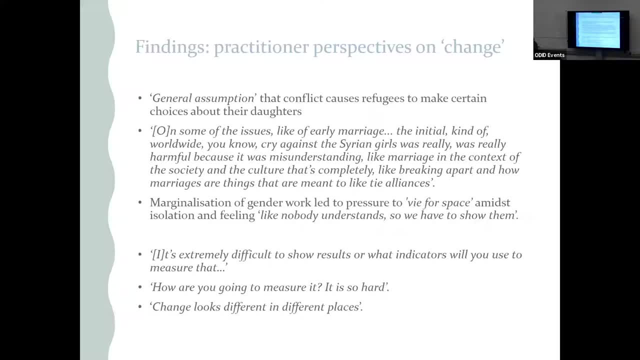 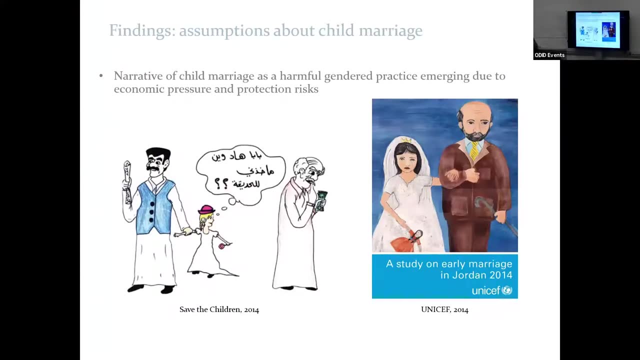 And so the first assumption is about child marriage And the fact that it increases gender displacement. So, in the context of the Syrian crisis, NGOs present child marriage as a harmful gendered practice That families resort to, largely for economic reasons And also to protect their daughters from harm. 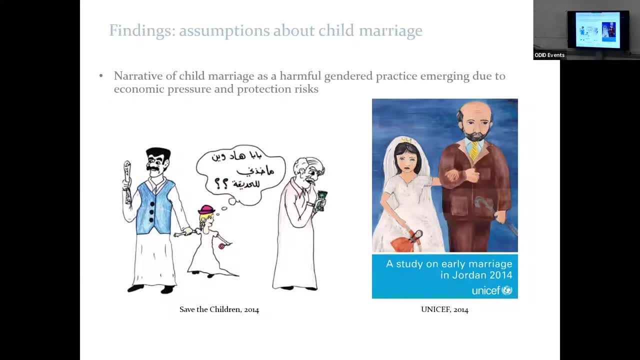 So the father is depicted as the decision maker Who's responsible for determining his daughter's marriage. So I think it's more true. in the image on the left, The father is saying: you know, Daddy, where is this man taking me? 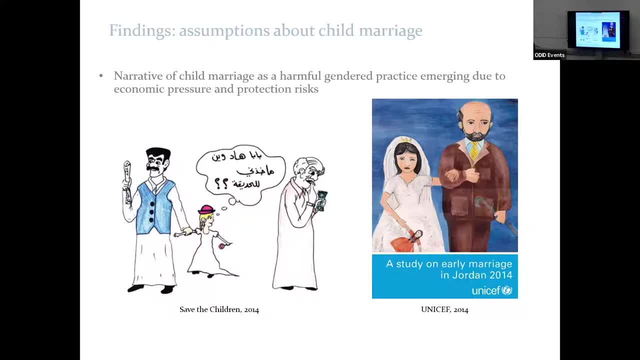 I'm going to the park, we're going to the park And then, scrolled at the man on the left, he calls it a marriage certificate. So humanitarian agencies tend to focus on this. They tend to focus on displacement as a cause of child marriage. 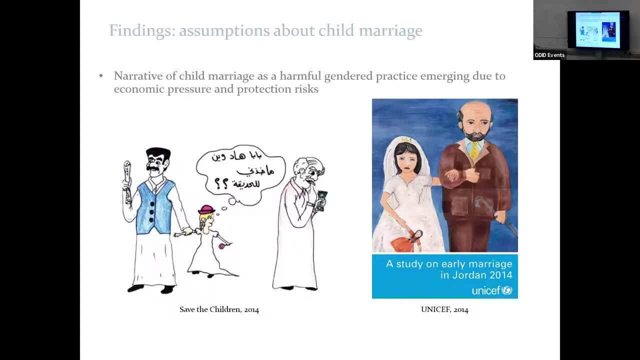 And this actually shifts the focus away from gender norms related to child marriage That prevent the conflict. It's one of the areas of displacement that comes later and causes this new practice, And this can neglect not only the social meaning behind marriage practices, Which one of the practitioners has talked about. 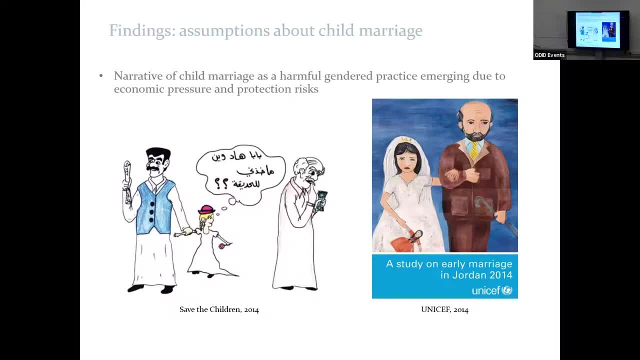 But it also limits how girls and men's agency and autonomy are depicted. So my research included life history interviews with women who were in their 50s and 60s who married as children, And child marriage for them was a cultural practice, not necessarily an economic one. 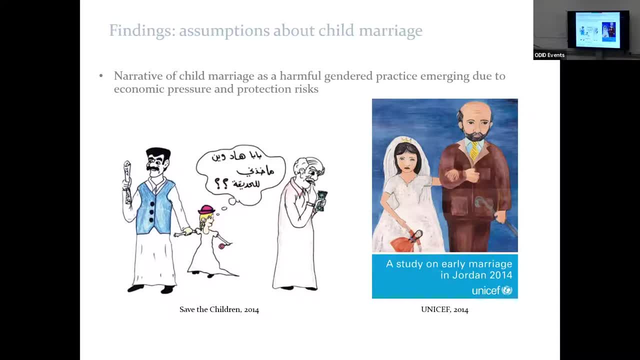 But a practice that was based on norms of what was expected for women, And there are also cases where child marriage might be the explicit desire of girls themselves. So one woman who was married, one woman was married at 17. And she had a husband who was a few years older than her when she was a teenager. 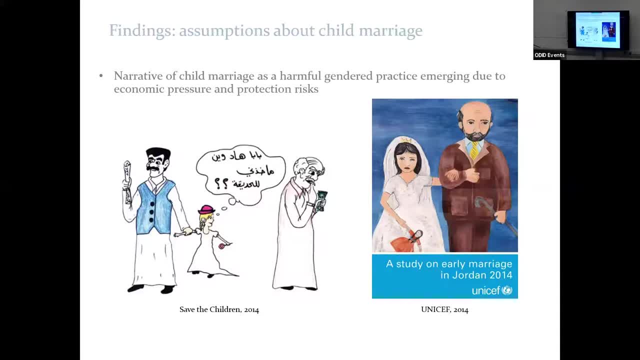 And was directly pursued by him And her father initially didn't agree to the match Because he felt, firstly, that she was too young to get married And then, secondly, that the prospective husband was a stranger Rather than a family member. So in some Western communities it was, and still is, customary to marry a family member. 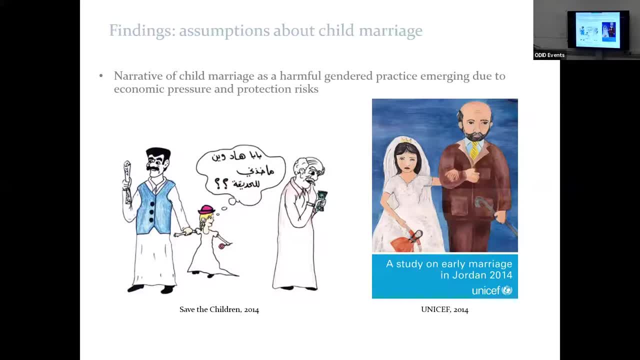 So usually a cousin, And so her prospective husband sent love letters to her for a few years Until her father finally relented And allowed them to marry, And she interestingly used this resistance from her family to get her future husband to do what she wanted. 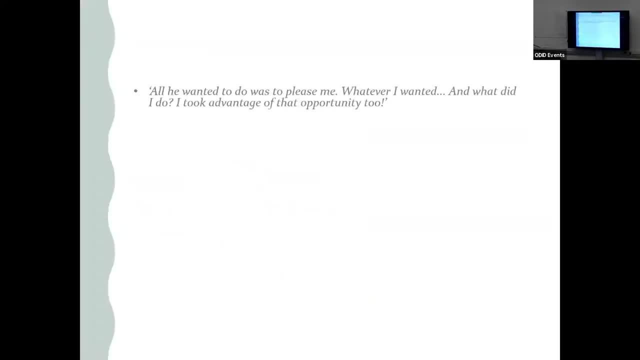 Even after they were engaged. So, speaking of her then fiancé, she said All he wanted to do was to free me. Whatever I wanted, And what did I do? I took advantage of that opportunity too. So, although she wasn't technically allowed to be alone with her fiancé, 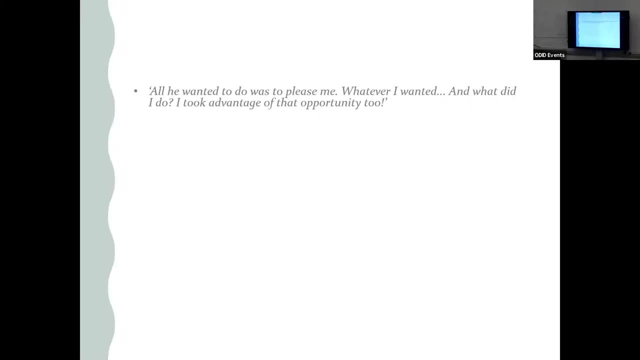 She worked around it. So she used his love for her to make him agree to secret meetings. And when they got engaged- because she didn't want to live with her mother-in-law As was customary, She persuaded her husband to make sure he was married. 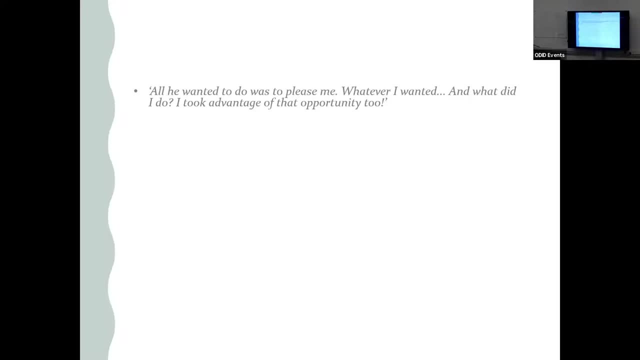 Defying the stereotypical image of a victimized girl who is forced into marriage. She used her own strategies to achieve what she wanted: To get married. Her family didn't push her into marriage, But she said that she wanted it, And she was even able to take advantage of the resistance from her family. 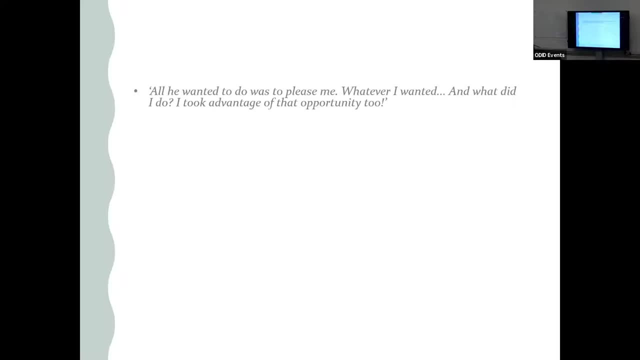 To get what she wanted out of her fiancé, And this was strategic. So it enabled her To accept power over him And she said Quite proudly That she continues to get whatever she wants from her husband, Even now, in her late 50s. 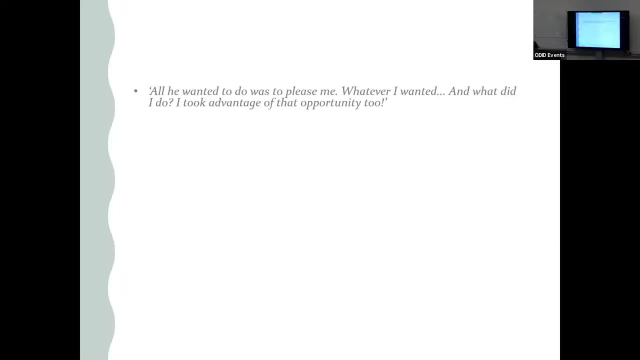 So during my interviews with her, While I observed her sort of issuing orders to various members of the family And telling them to bring this, Take this, Go and do that, She also gave examples of how her husband does. whatever she wants, She tells him where to go. 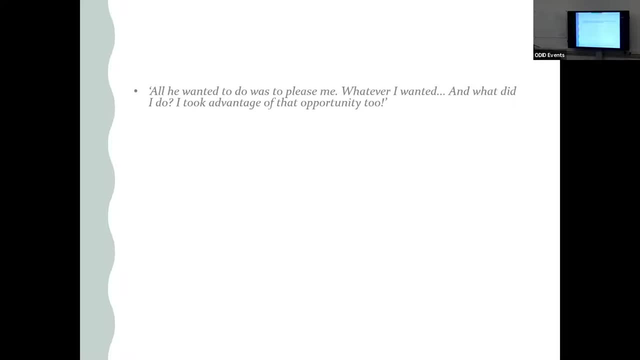 Where not to go, And this is how their marriage is. Just as young girls and young women may choose marriage, They can also reject the pressure to marry, And I think understanding that girls have this ability to refuse Also disrupts the singular narrative about humanitarian. 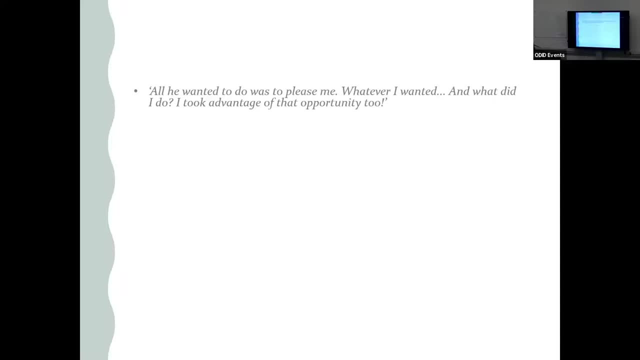 About Syrian marriages That humanitarian actors sometimes perpetuate. So one male research participant Explained how he fell in love with a girl when he was a teenager in Syria And he would send her love letters. But she ripped these up And she told him that she wanted to finish secondary school first. 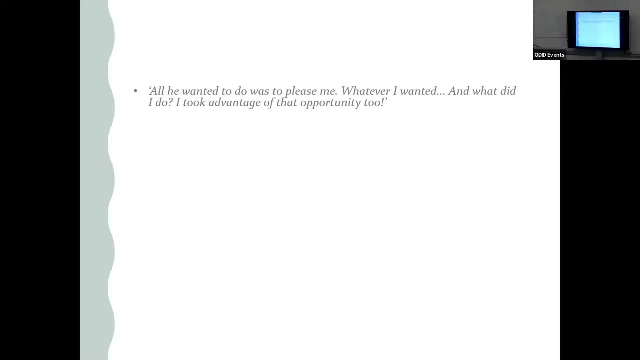 Before marriage: Another woman, who is now 21 and unmarried, Is seen by her extended family as a spixter, So they are shocked that even in Jordan She has refused prospective suitors. But she is a spirit And so she goes. 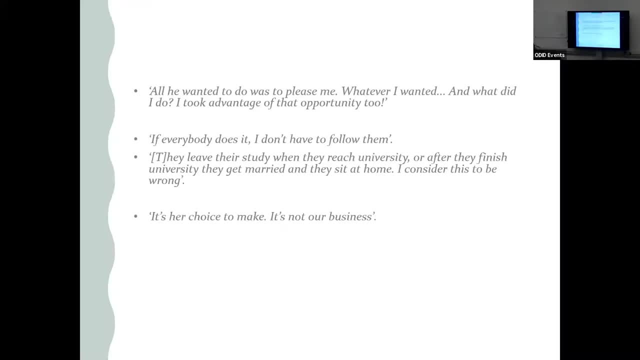 If everybody does it, I don't have to follow them. She also said that she has. She also sees marriage as something that stops women from being able to use their skills. So she said, you know, They leave their study, they reach university, but after they finish university they get married and then they stay at home. 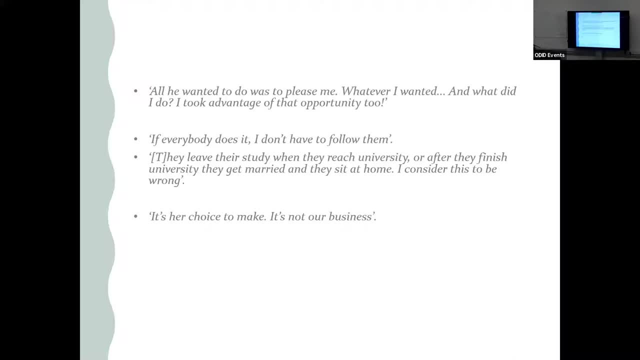 I consider this to be wrong. Her parents are very supportive of her decision to study, and her father himself is a professor whose education focus has influenced her life. Singular narratives about child marriage may also be disruptive when we consider the reasons for marriage across the life course. 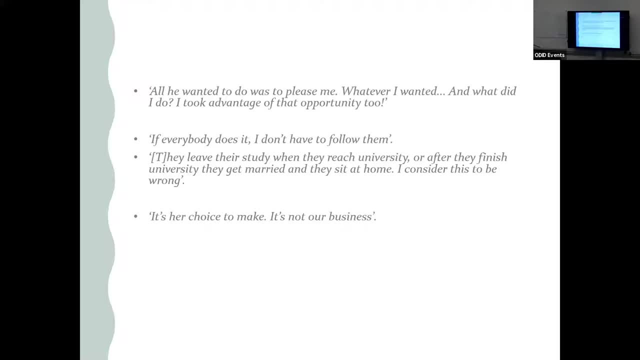 So older women, for example, may also choose to get married. choose not to get married, sorry, when they face economic pressure. So one older woman became a widow at age 29 in Syria And although she struggled financially, she refused to remarry. and she remains single now, in her early 60s. 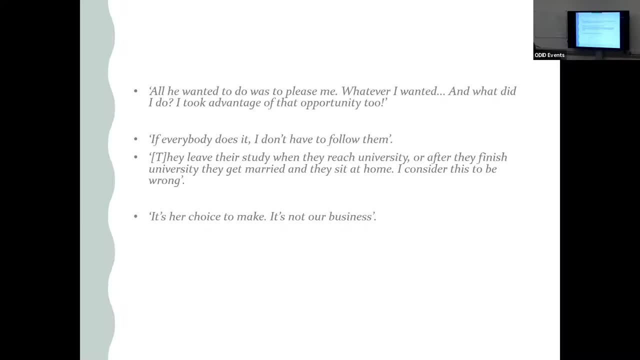 And when approached by suitors after her husband died, her family told them: it's her choice to make, it's not our business. She said that she had agreed with her husband That if anything happened to him, that she would not marry again. 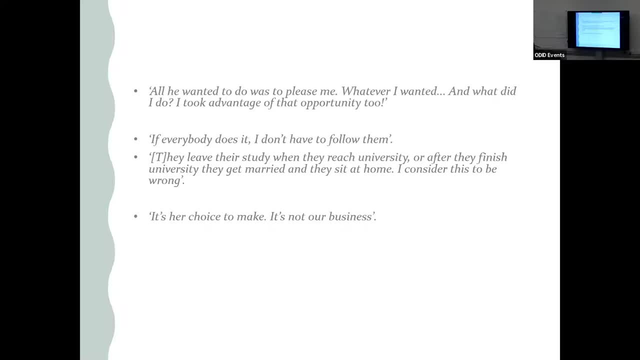 And also felt that second marriage would result in her not seeing her children as the new husband's immediate. So this is an example of how, even when facing economic pressure or the need for male protection, women may not necessarily be driven to marry, Which is a different way to how humanitarian actors typically talk about marriage amongst Syrians. 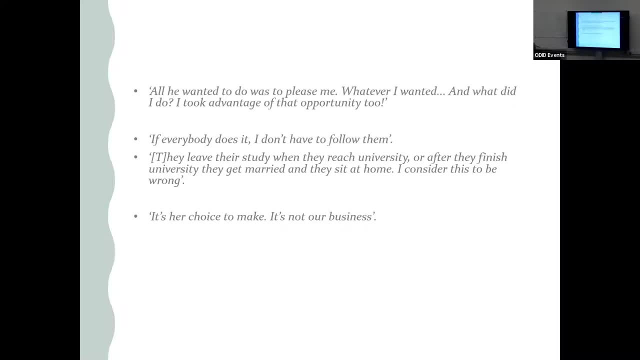 Her relatives did force marriage, but they allowed them to make a choice which would also be tied to their age and the relationship with women. Importantly, sometimes a marriage can restrict rather than increase options, In this case potentially limiting her ability to care for her children. 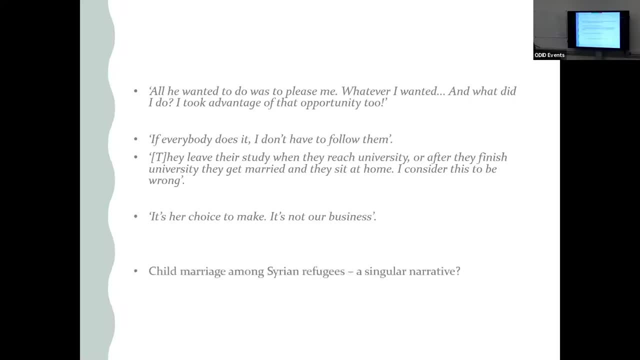 So these brief examples help to illustrate that the practices of child marriage are not necessarily uniform. It's difficult to generalise And there's not a singular narrative of how Syrian marriages occur, And this is why it happens In the case of Syria. we can't necessarily pinpoint and say: well, economic pressures resulted in. 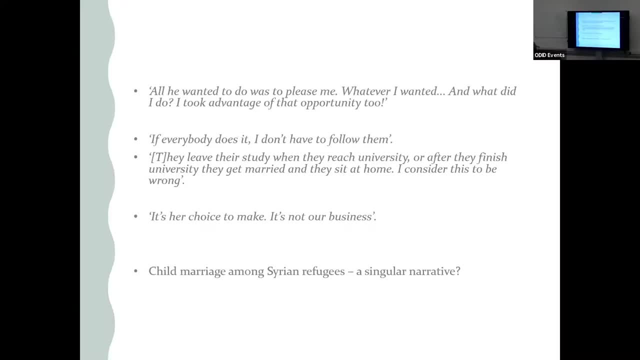 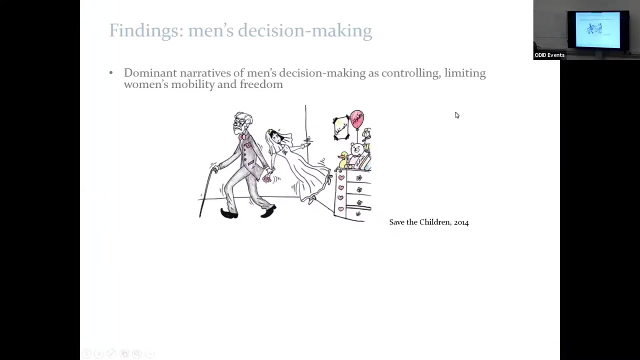 in in child marriage emerging as a practice, Because in the case of Syria there is a lack of data on child marriage before the war, And so that makes it really difficult to draw conclusions about the practice during displacement. So the second assumption about change relates to men's decision-making about women's lives. 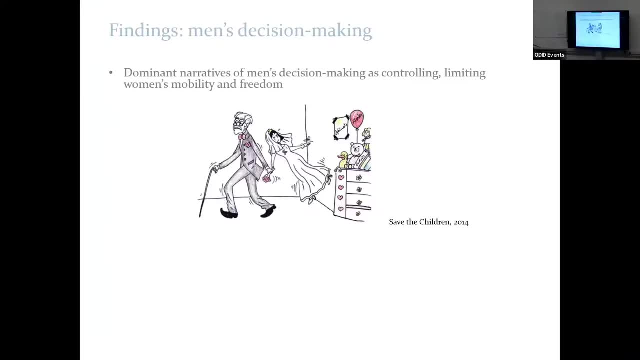 So humanitarian reports discuss how, as a result of displacement, men can become more controlling, limiting girls and women's mobility and preventing them from accessing education, work or socialising. So, in contrast to the overwhelming negative portrayal of Syrian women in humanitarian agency reports, 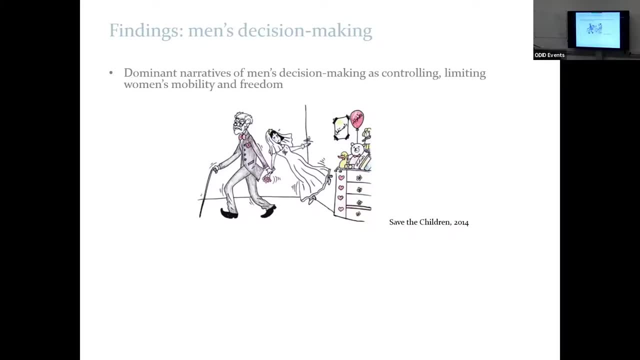 the Syrian women I interviewed shared quite different examples of how men in their lives have supported them and been quite encouraging. So one woman who is now in her mid-thirties stopped attending school after the ninth grade because her new house was too far. 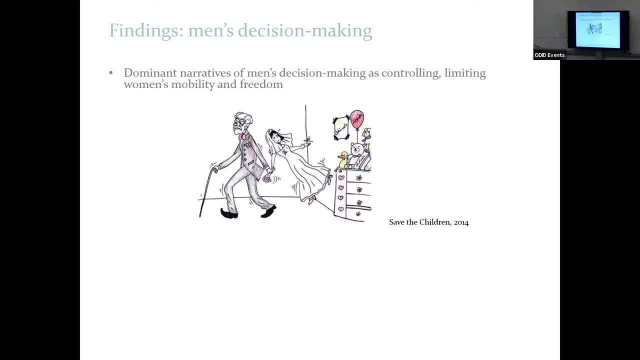 her new school was too far from her house And she wished that she continued studying after marriage And in Jordan. she told her husband this and she recounted this conversation with her husband. He told me: if you told me you wanted to continue, I would let you continue, but I didn't tell them I wanted to. 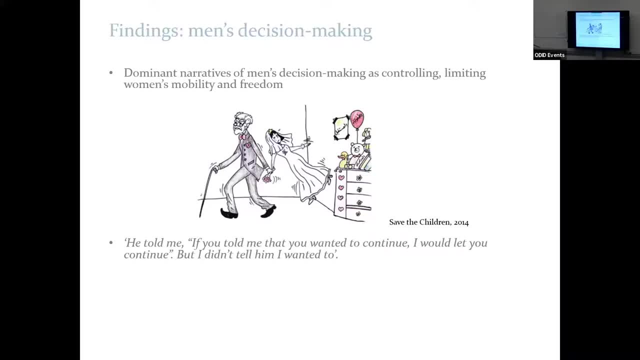 In Jordan. her husband had encouraged her to continue her education and at the time of the interview she was considering this. One woman who I mentioned earlier, who has refused multiple students, described her father as her role model. She's a professor who has encouraged her in her efforts to continue studying in Jordan, even when she decided to change her major to a less prestigious one. 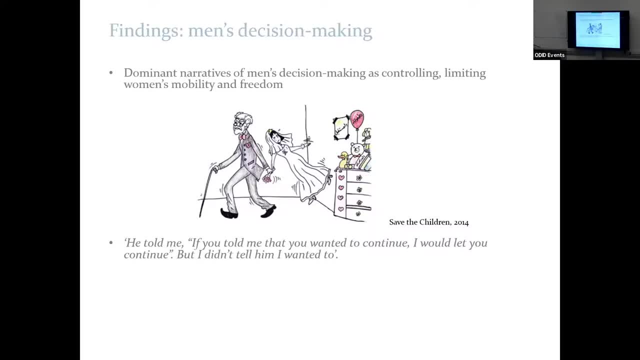 Another young woman, whose father was a businessman in Damascus, explained how her father took them to book exhibitions and galleries, using these as learning opportunities. His influence now drives her to continue completing her studies. So in these two examples, Syrian men were actually quite positive forces in the lives of their daughters and their wives. 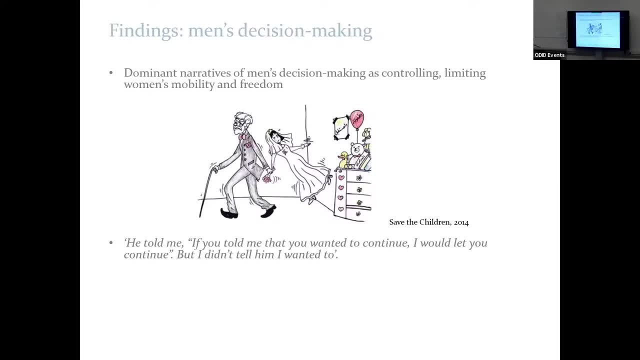 For a 19-year-old woman who wanted to continue her education after arriving in Jordan, the biggest challenge was not her husband, but actually her in-laws. So she married a Syrian man after arriving in Jordan and became pregnant, And then, when she had a baby, she wanted to continue studying, but her in-laws raised objections. 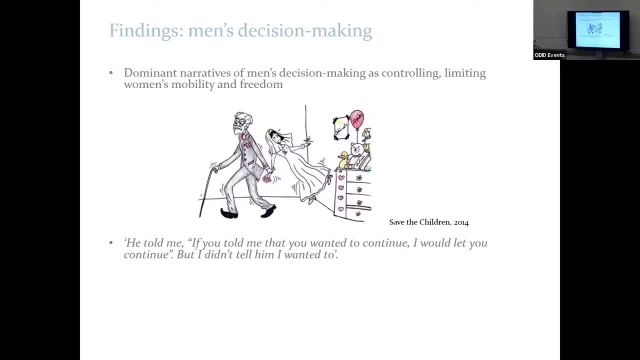 So they were concerned that she wouldn't be able to manage her household as well as her new child and study. But she was able to navigate these objections by proving she could still complete her studies. She said they found in my house: I wake up early, I study early, I do my house, I cook and then I finish. 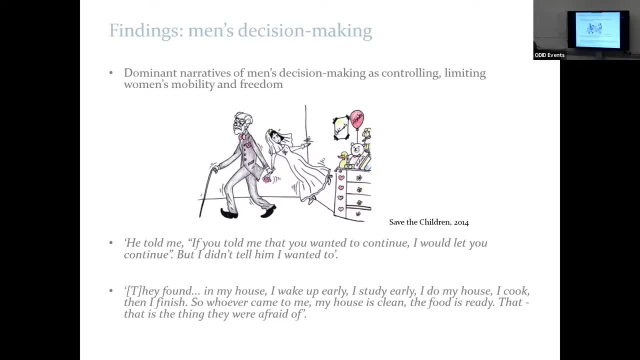 And, if it ever came to me, my house is clean, the food is fresh. That is the thing that they were afraid of. In this case, it was through affirming what we might call traditional gender norms that she obtained what she wanted. 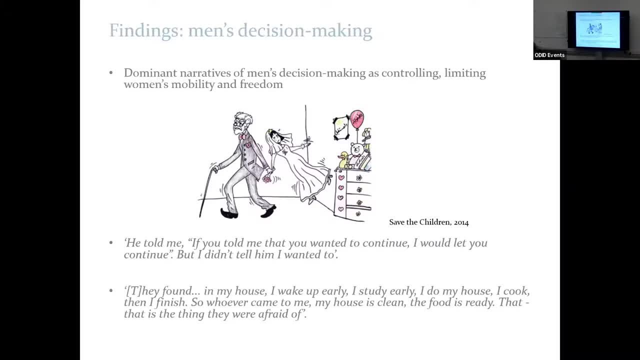 So she resisted one norm that said women have to continue studying after marriage, by invoking her ability to meet gendered expectations in another area, So completing her caring duties, And she was able to bargain with her family and choose what was most important to her, which was her education. 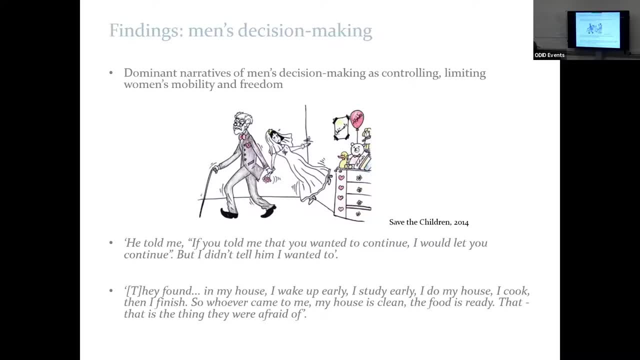 So, like her, women may also choose issues that they had time to acquiesce on in order to get what they wanted, And, like her experience, it might not always be men who make decisions for women, but the role of the broader family, and especially in-laws, is one that needs exploration. 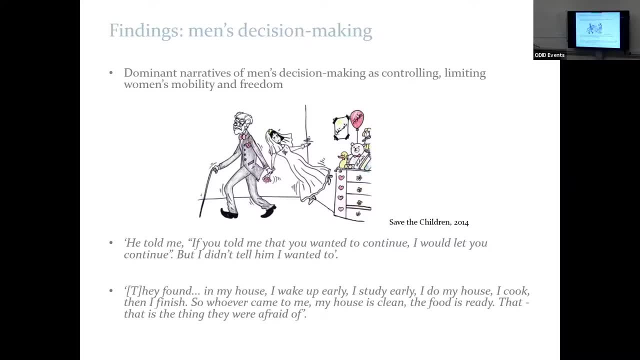 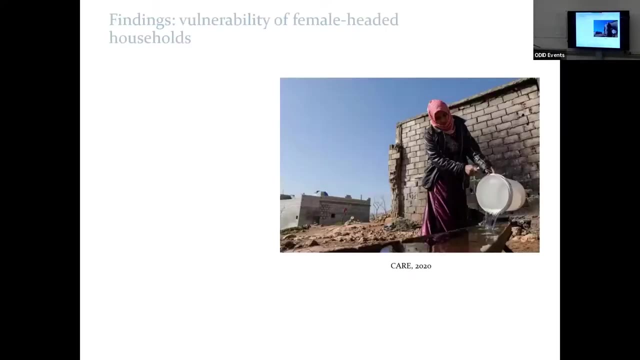 Even when family members are struggling, women are always there to help. They are there to protect and accept control. There may be opportunities to manoeuvre around these expectations and for women to still get what they want. Men may not necessarily have the final or the earliest word. 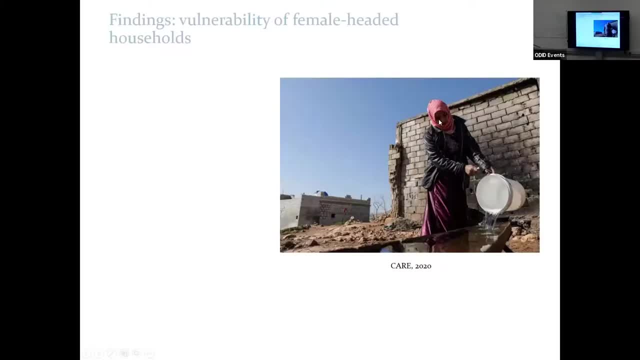 And the third assumption is about the vulnerability of female family members. So, according to humanitarian actors, household structures change and there is not necessarily conflict Resulting in families being torn apart and women being forced to live alone for the first time. 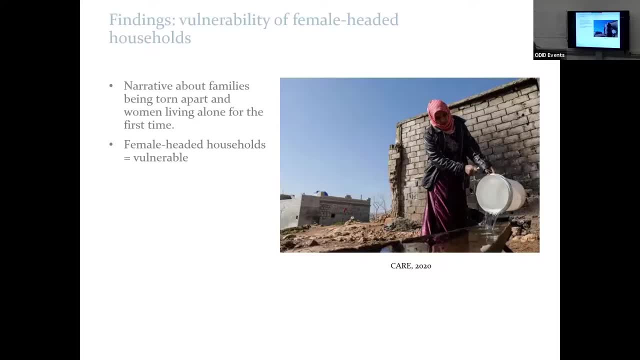 And households are, according to these reports, female-headed and therefore vulnerable deserving of specific assistance. Being female-headed is one of the criteria that many agencies in Jordan and in the region cannot determine if refugees are eligible for cash assistance. So back to the point about the need to consider norms before displacement first. 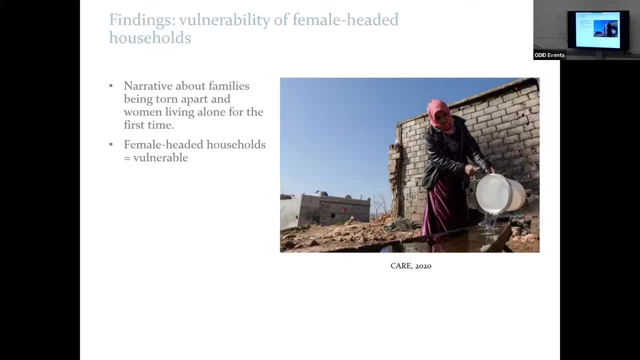 It's really important here to think about the history of the region. So from the 1970s, Syrian men would leave Syria and go to the Gulf for economic opportunities, And this historical pattern of economic progression was also evident from participant accounts. 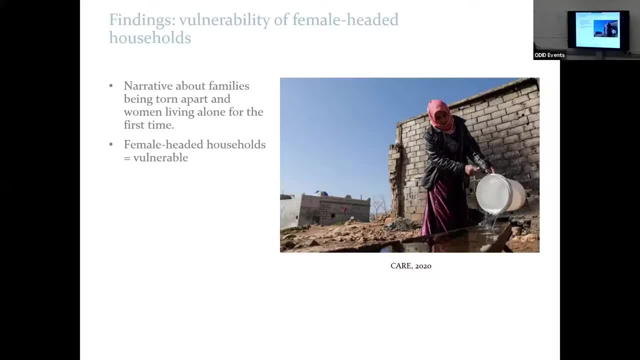 The one Syrian woman explained how, one by one, her older brothers left Syria to work in Saudi Arabia because of better economic opportunities. Now the older woman said that her husband worked in Saudi Arabia for several years, returning only in the summer, while she remained in Syria raising her young children. 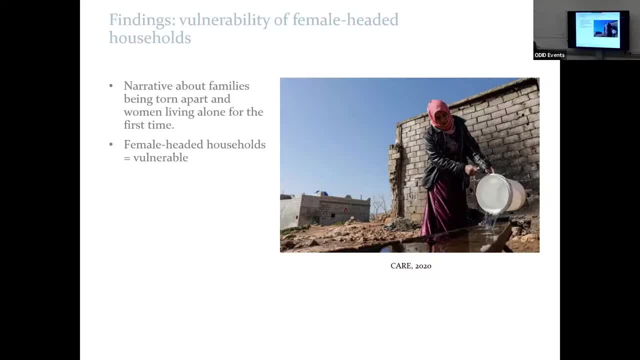 Another man said in an interview that he was away from most of his children's childhood and early adulthood, visiting only every summer. The displacement is not necessarily the first time that women have been head of households. Many Syrian women shared that they were responsible for what they called men's tasks in Syria. 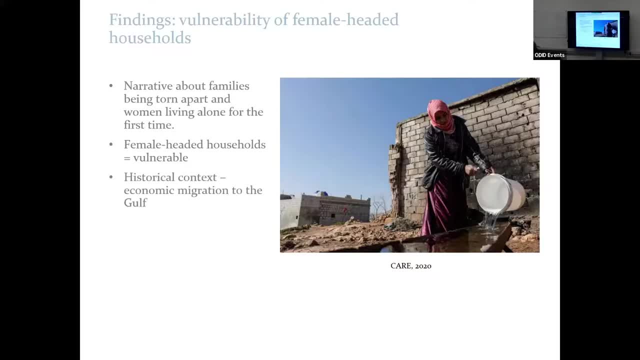 or their husbands or their fathers were absent. However, even having absent male family members didn't mean that women were alone, because they had support from extended family members, which are an important fixture in Syrian society. Many women discussed how they had support from extended family members in caring for their children. 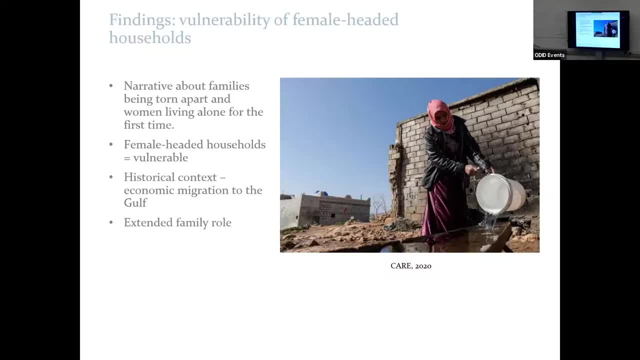 and in managing their household, both in Syria as well as after coming to Jordan. So, in contrast, humanitarian narratives emphasise women's vulnerability, especially the challenges faced by female-headed households, What is assumed to be vulnerable by default, And this is, I suggest, linked to the way female-headed households have been positioned in other emergencies. 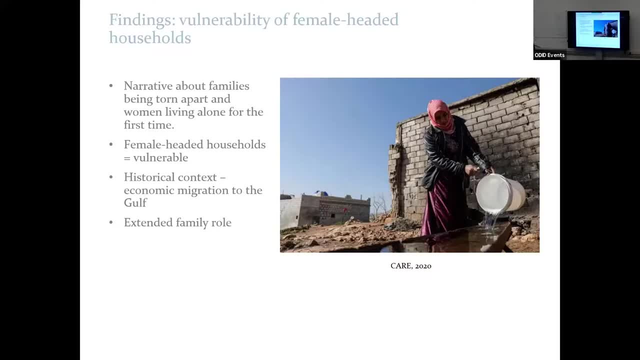 especially in the context of African emergencies, and that sort of narrative about female-headed households has been transferred into the Syrian context. And these narratives are often based on assumptions about refugees' lives, but they have direct implications for humanitarian interventions, So they can result in certain groups being prioritised. 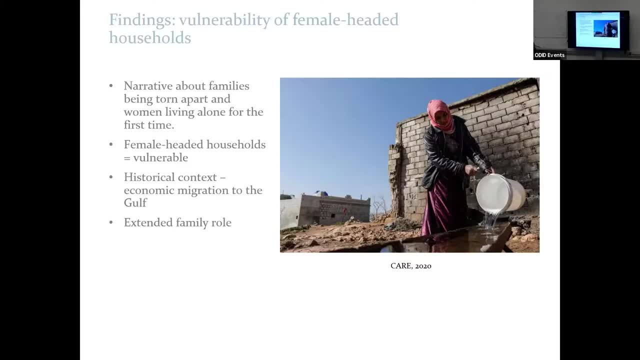 over others in receiving aid or in paternalistic attitudes towards certain groups of women. So female-headed households, for example, are assumed to be automatically disadvantaged. So there's little recognition of women's autonomy, their decision-making or their existing social capital. 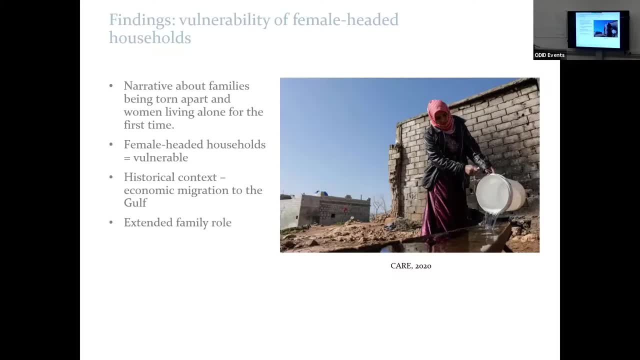 These women are assumed to experience not just gaps in economic security, but also low awareness of how to care for their children, how to protect themselves and what their rights are, which is where their dreams come in. This kind of narrative affirms the role of humanitarian actors. 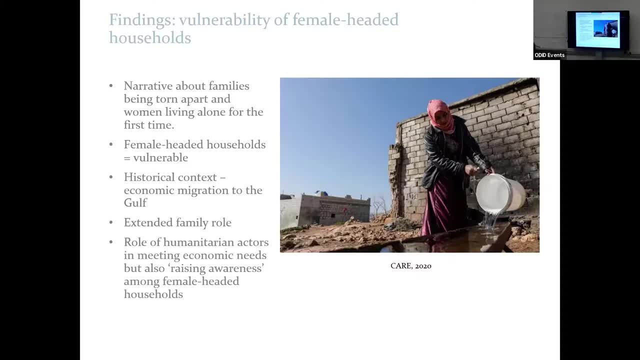 in raising awareness justifying future funding. The problematic assumptions underlying these conclusions are not necessarily questions that we interrogate in films. Instead, it's attuned that humanitarian actors know what they need to know about people's vulnerability in order to respond. Syrian women may already have some of the coping strategies. 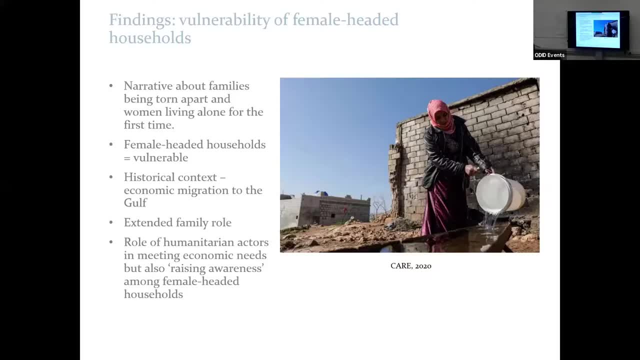 and the abilities to adjust to different household structures. So it's not as simple a case of displacement in the trigger that disrupted family life, because some of these disruptions have already been happening. This is not to say that female-headed households are not vulnerable. 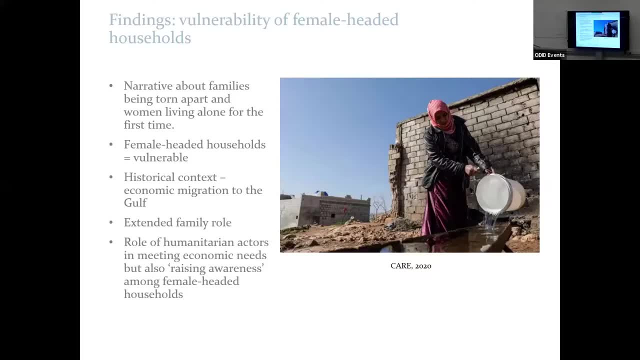 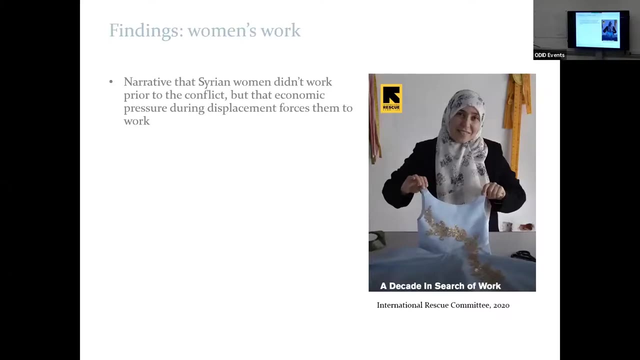 but it's more about raising a question about whether we should automatically presume vulnerability. Okay. so then the fourth final narrative is about women's work. So a common humanitarian narrative is that Syrian women did not work for foreign law, but they remained in the home. they looked after their children. 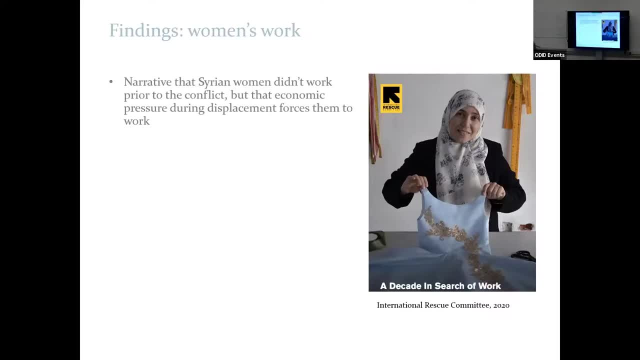 they cooked, they cleaned their houses and during displacement. the narrative has shifted. So humanitarian agencies say that, because of economic insecurity and because of pressure on the family, women are now forced to work And humanitarian actors exercise their role in supporting women in developing the skills and the knowledge so that they can be productive actors. 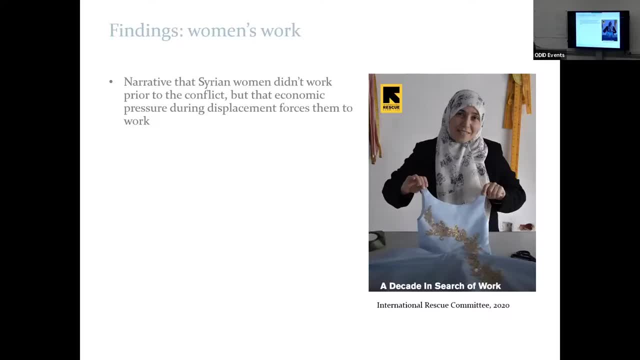 So my research found really quite mixed experiences. There was a mixed experience of work both before and after displacement. So before displacement there were women experiences that really challenged this idea of culture or tradition automatically stopping women from work. So some women only worked before marriage. 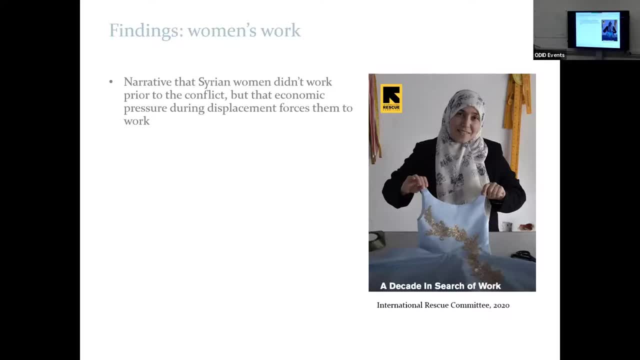 while others continued working after marriage. for example, It wasn't always the case that the husband stopped the wife from working. Sometimes the woman decided to stop herself. Sometimes the family encouraged her to work. So one woman: she ran her own clinic and worked at a government hospital even after marriage. 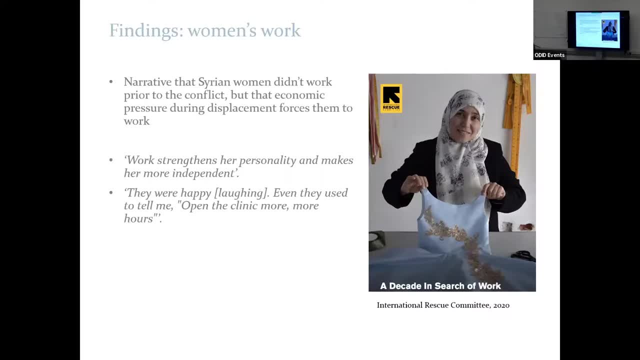 And for her. work was a positive thing for a woman, She said work strengthens her personality and makes her more independent, And she thought her years studying in the medical field would be wasted if she didn't work. And, interestingly, her family also encouraged her to work. 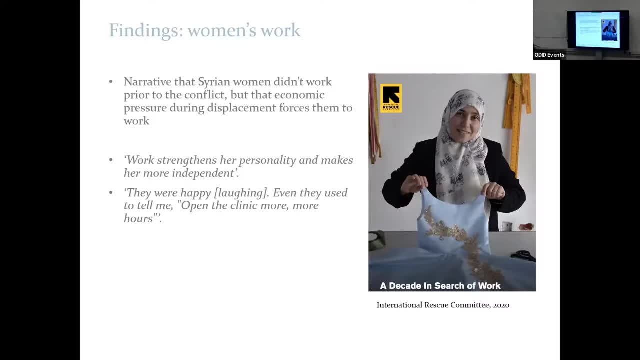 So she said they were happy. Even they used to tell me open the clinic more, more hours, And this is likely due to the high level of education of both her husband and her father. Their support helped to create the conditions for her work. 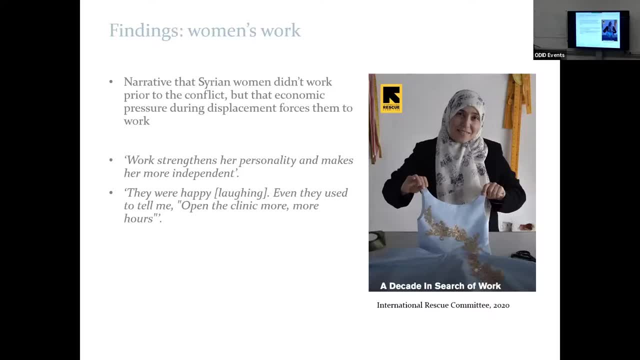 A few women talked about how it was acceptable for Syrian women to do that, Which is not that unusual because we know that Syrian women who have family property. they were involved in trade and business even from the Ottoman world. However, multiple women attached conditions to their work in Syria. 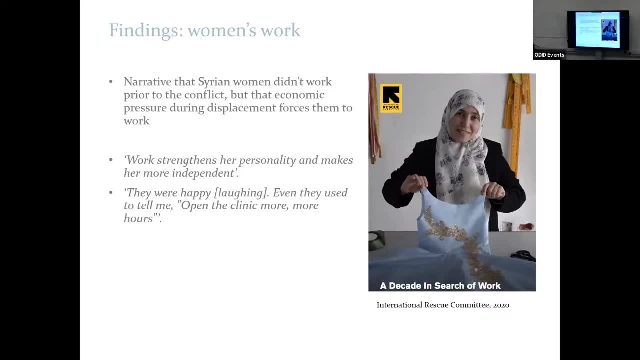 They said it could only occur if a woman was still able to manage her household responsibilities. So one woman said a woman is not forbidden from work as long as she doesn't cut through her home. For some women, financial pressure meant that they needed to work. 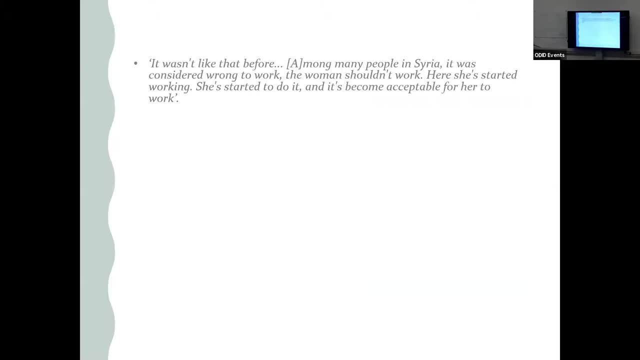 And I said one woman said it wasn't like that before, Among many people in Syria, it was considered wrong to work, That women shouldn't work Here. she started working, She started to do it and it's become acceptable for her to work. 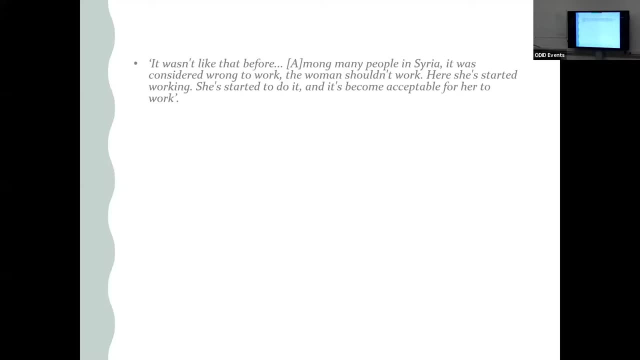 One woman told me she secretly works so that she can pay for basic necessities Like taking out of the house and doing work in other people's homes, cleaning and running errands without her husband knowing. For another woman, work is also something that the husband is not happy with. 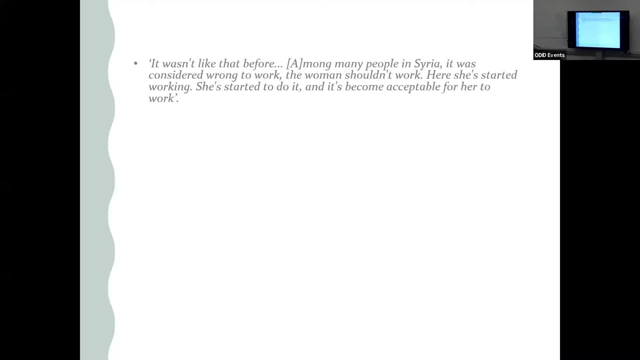 So one woman from Damascus who married another Syrian after she came to Jordan said that when she goes to NGO buildings for different activities or for awareness raising activities, her husband will always tell her. he keeps telling me cover, cover. So how can I go out to work? 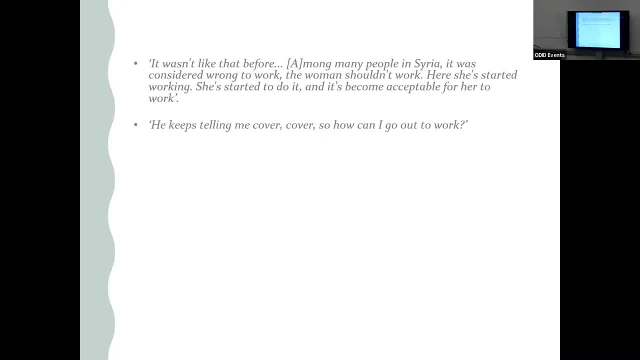 For others, working in Jordan is something they were able to negotiate with their husbands, which was made easier by necessity. Another woman, whose family is quite conservative, felt that the issue was the type of work that women needed. She said I wish that the women would work to support her husband. 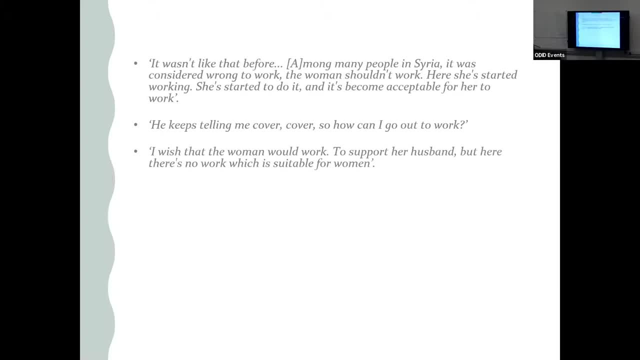 but here there's no work which is suitable for women. One woman thought it was an exceptional situation that the man was not able to provide and therefore this made it possible. She said: then that's a possibility, She will be the man and he will be the woman. 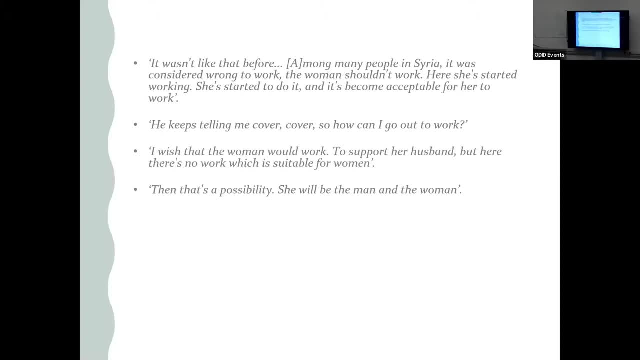 She will be the man and the woman, And this really came up quite a few times in multiple interviews, where women talked about how, when they were doing their jobs, they were the same as well as the woman. Other women referenced this change when they talked about taking responsibility outside the home. 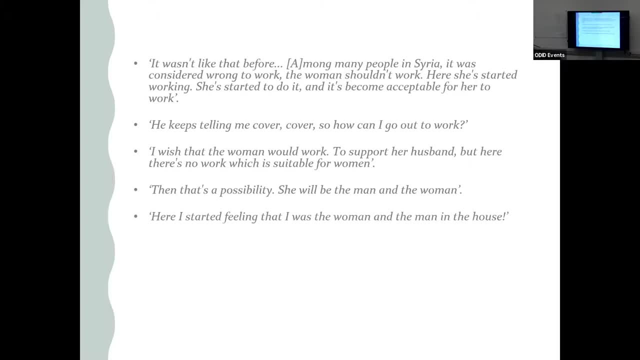 Here I started feeling I was the woman and the man in the house. One comment from a Syrian woman illustrates that working inside the home is sometimes not seen as real work or real responsibility. So one woman said: now it's me Yanni. this means now I'm the responsible one. 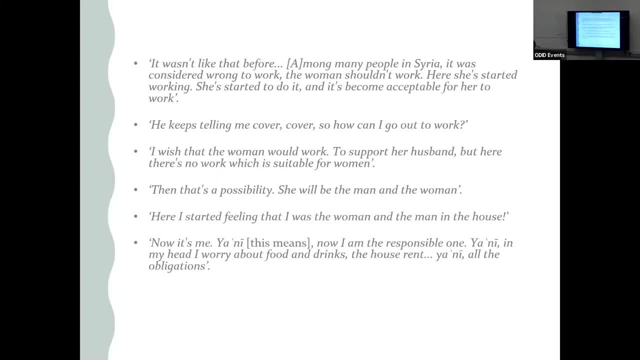 This means, in my head, I worry about food and drinks and house rents. This means all the obligations. Taking on tasks that were previously men's responsibilities caused this woman to refer to herself as the responsible one, as if the tasks she completed before were not real tasks. 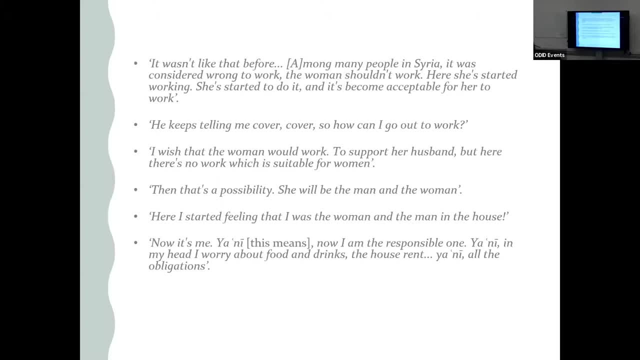 in comparison to paying the rent or budgeting. This comment can be argued to be reflective of prevailing perceptions among some Syrians, as well as humanitarian agencies, that the work done before displacement was not real work compared to the tasks they've taken on during displacement and especially compared to economic activity. 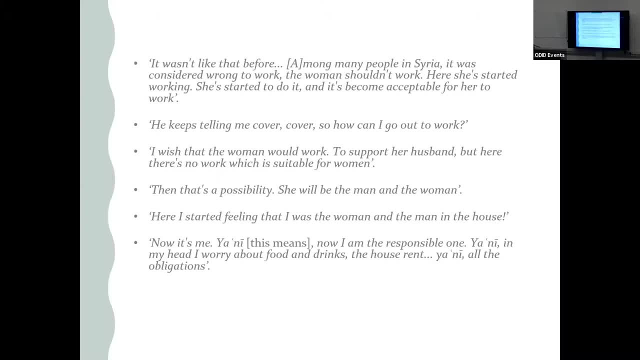 Although gender and feminist activists have spent years trying to emphasise that women's so-called reproductive work inside the home is just as important as productive work which generates income, in reports issued by humanitarian actors, we see this influence of neoliberal ideas. It makes it appear that women who care for children 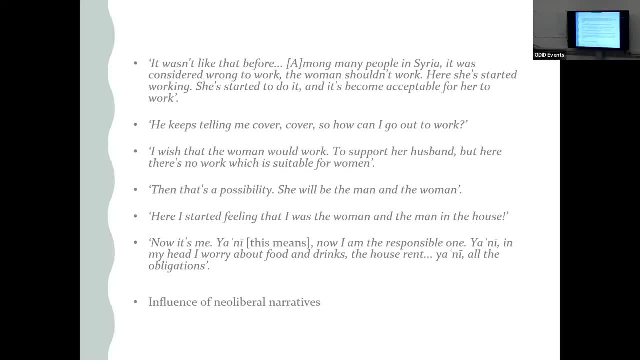 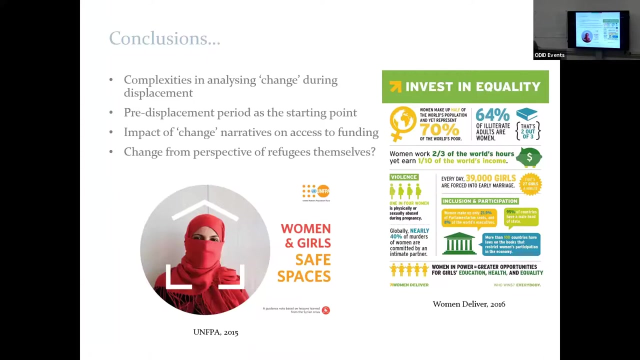 and income from household tasks are disempowered by default, And so, within these narratives, it seems that to truly be considered empowered, a woman must do everything. As I remark, there are still questions about the relevance of this concept of change within narratives about refugees and gender. 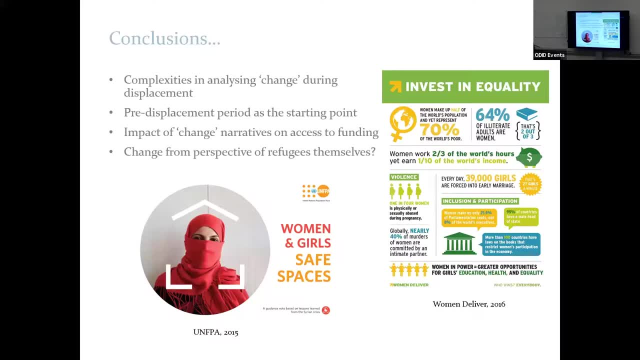 The examples I've discussed today in relation to child marriage, men's decision-making, family and household and women's work demonstrate some of the complexities in keying down gender norms during displacement and especially in making statements about changes that have occurred as a result of displacement. 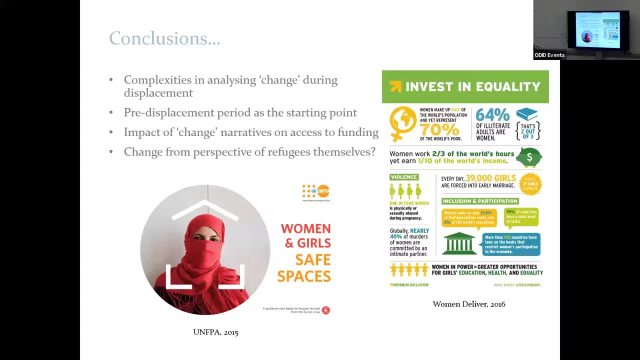 Humanitarian agencies have typically engaged with issues of gender change among refugees by speaking of change only with reference to the displacement period instead of before displacement. Focusing analysis on the displacement phase means that the pre-displacement period becomes synonymous with tradition and culture, which Leila Abu-Lughod argues means not just flattening cultures. 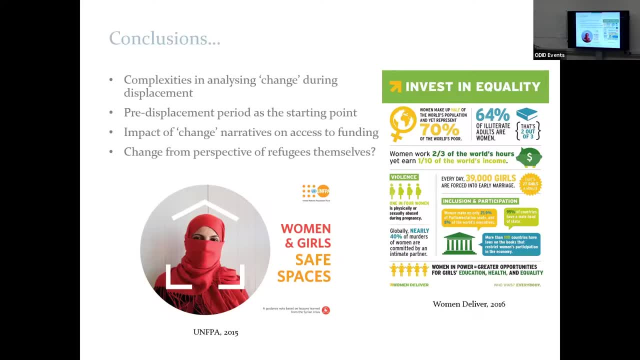 stripping moral systems of their complexity, it means erasing history. When tradition and culture are invoked in the name of gender analysis, it results in stereotypical tropes and judgements, presenting refugee experiences as fixed, homogenous and opposed to modernity. 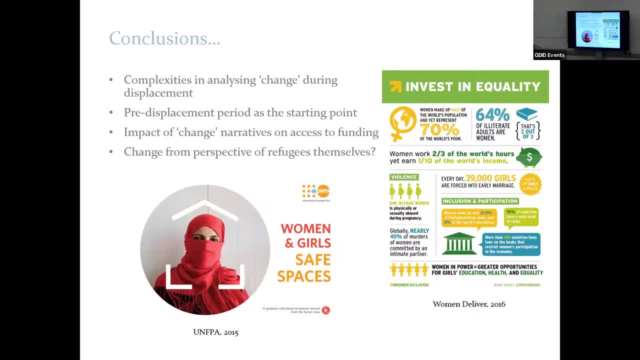 And for humanitarian actors, who sometimes appear fixated by the idea of capturing changes in gender norms through displacement, it's critical to recognise that change can't be understood unless the starting point is clear. So assuming a pre-set conservative cultural mindset can negate differences in belief systems and agency between individuals. 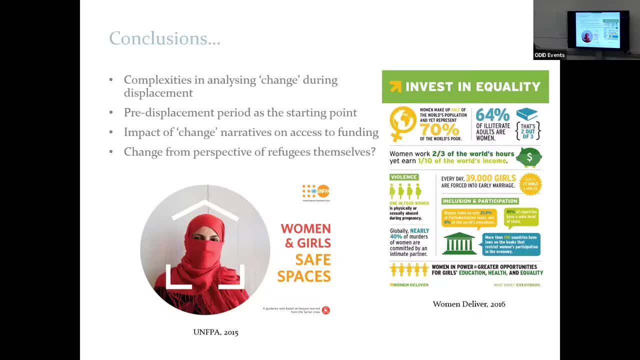 neglecting the very starting point is a key point for gender norms. Indeed, many refugees may already be empowered, But sometimes prescriptive approaches to empowerment assume zero baseline knowledge, and so the focus then becomes on raising awareness. The reflections of humanitarian workers on change. 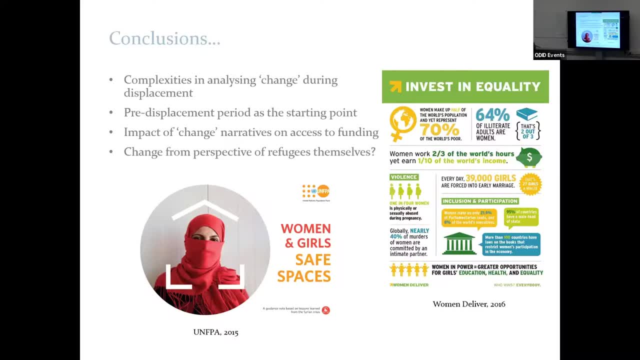 highlight quite complex motivations in the assumptions made about displacement. When humanitarian actors present analysis of gender changes during displacement analysis is not necessarily neutral. Employing the rhetoric of change in the context of displacement brings attention and more significant refunding to the much-neglected programming sector of gender equality and women empowerment. 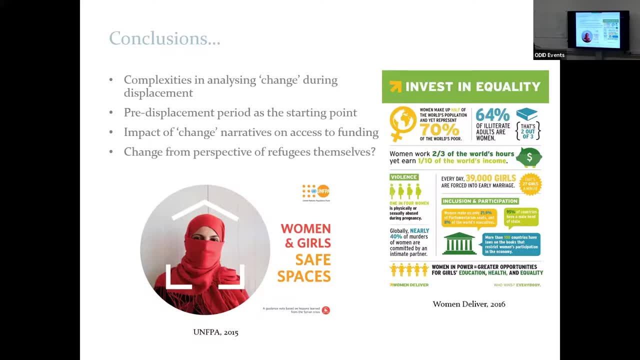 Working on such programmes have a vested interest in emphasising narratives that make funding possible. Making the case for why gender should be prioritised within the humanitarian sector can quickly become about gathering the most sensational and compelling examples of women's oppression, What Andrea Cornwall refers to as gender myths and feminist fables. 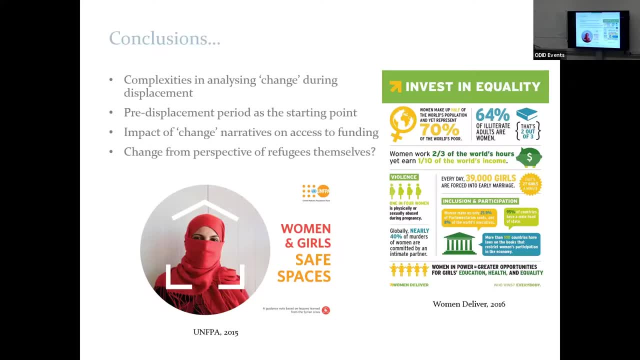 can then take the place of real analysis. Refugee lives may become reduced to tantalising tropes operating as clickbaits to try and generate interest and funding. Humanitarian actors then present their roles in transforming refugee lives and addressing these oppressions, mapping out the changes they will achieve. 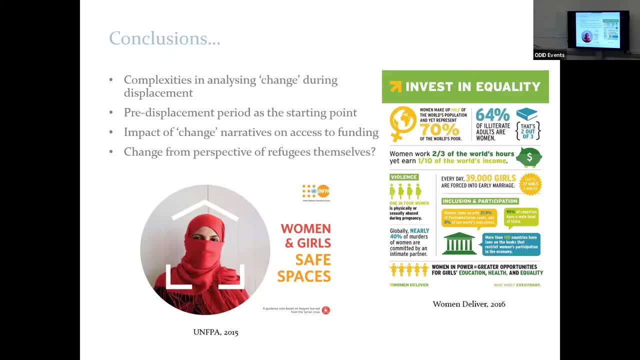 to meet logframes and theories of change, While humanitarian actors increasingly rely on universal quantifiable indicators. this misses the fact that change means different things to different people. Rarely is the focus on change from perspectives of refugees themselves. Instead, others make judgements about their lives. 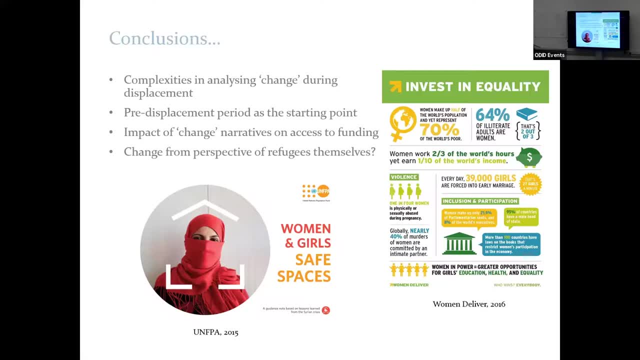 So how can humanitarian actors and scholars and activists actually break in with this concept of change And how such debates and assumptions actually lead to change? The late Judy Earl Bushra suggests that need to actions may not always be possible, And she recommends that we reflect on a few key questions. 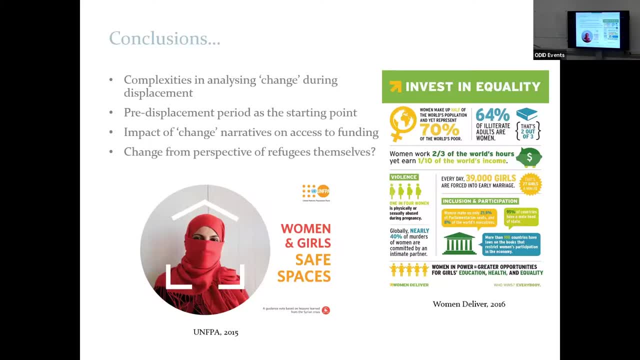 when we think about change. So I'll end with these questions that she suggests. She said: do people see their lives as being better or worse than before, And how far is the interpretation of this question coloured by their own gendered experiences? How far are the interventions of development or humanitarian agencies? 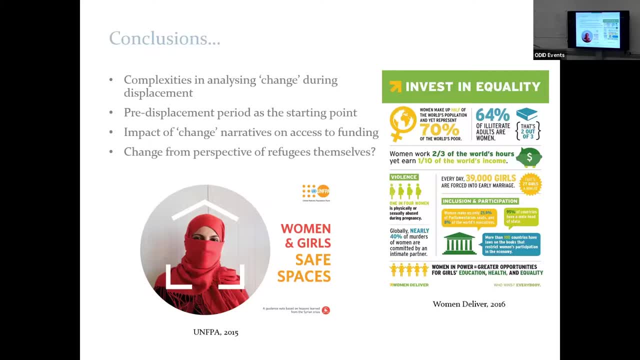 coloured by their own perceptions and values. Thank you. What I'd like to do is to invite any questions or comments or thoughts that you might have. We have about 15 to 20 minutes. I'm going to take three at a time. 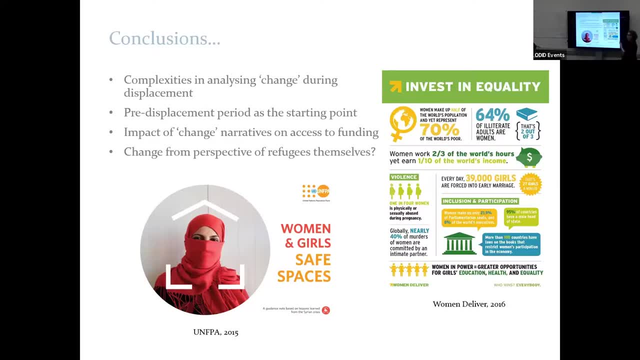 And if you could just introduce yourself to the speaker and then keep it as short as possible so we can have as many people in the conversation as we can. Who wants to start us off? Yes, Hi, thank you so much for your amazing presentation. 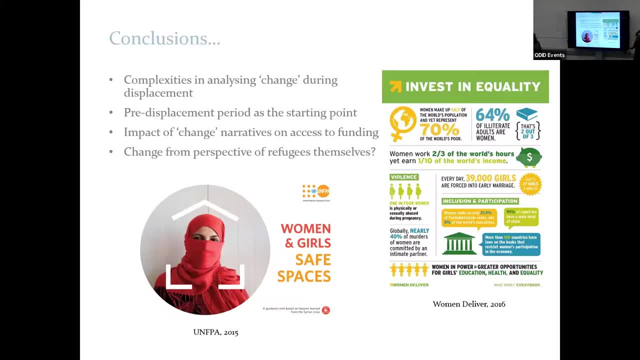 My name is Erin and I study global governance and diplomacy, And my question is: in your research, and in feminist research in general, how do you balance giving voice to people who want to share disturbing stories that might seem to confirm assumptions, without playing into dominant narratives that people have? 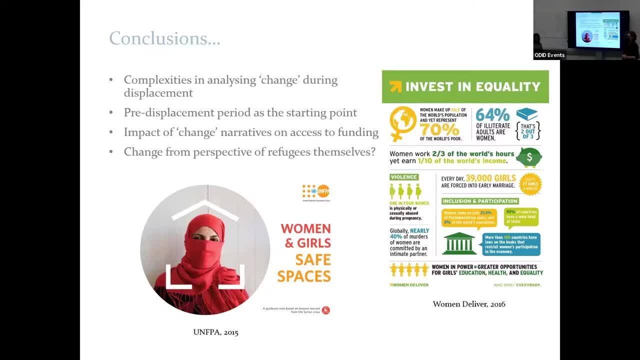 Hi, I'm Asma and I'm in the MNC of refugee, So I guess I'm just going to catch my question in an example quickly. So I so appreciate your thoughtful presentation And I have been thinking about if, say, we were to take an American woman or a British woman. 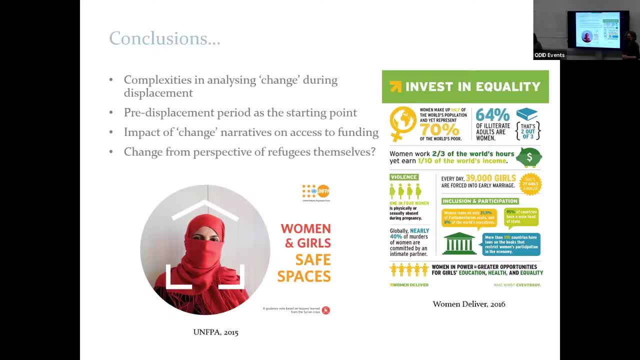 and talk about the relationship that she has with her father or her brother or other members of her family. it doesn't seem that we would attribute that to these larger realities of gender within their society as readily as we do when it comes to say: 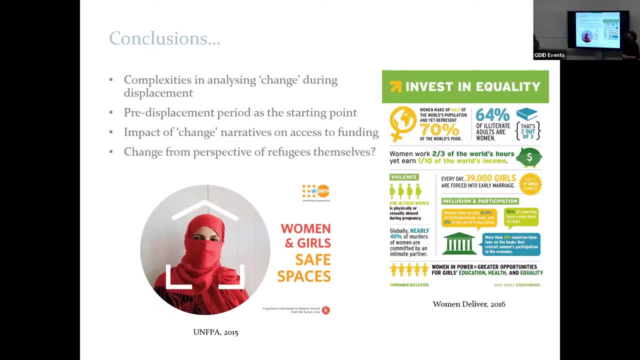 a Syrian woman's relationship with her father. So I'm wondering at what point you think in the future would we be able to get past the always-attributing personal relationships that refugees have with people in their lives to these larger narratives I have a follow-up question. 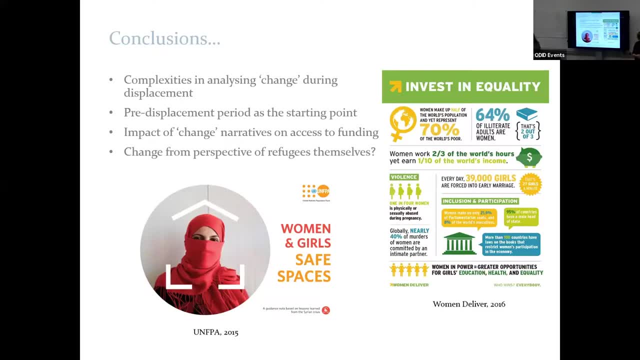 Yes, Thank you. Thank you so much for your presentation. My name is Sandra and I'm studying a Master in Public Policy, And my question is related to the collaboration that the humanitarian sector is having with other actors that are also important players in helping the empowerment of women. 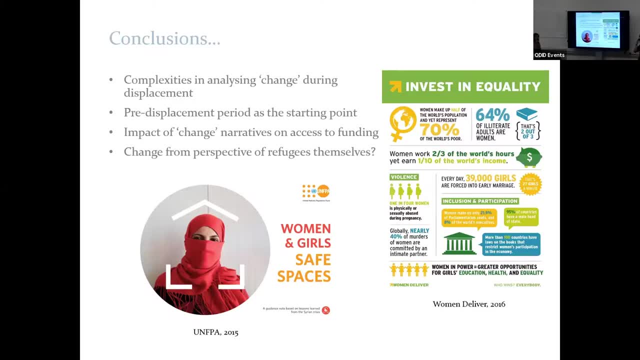 in refugee settlements, especially with governments or the private sector. Is there any example of collaboration of the humanitarian sector with these other actors? And yeah, thank you, Thank you. Yeah, thank you, Michelle. Yeah, yeah, sure. So the first question about sort of how to place 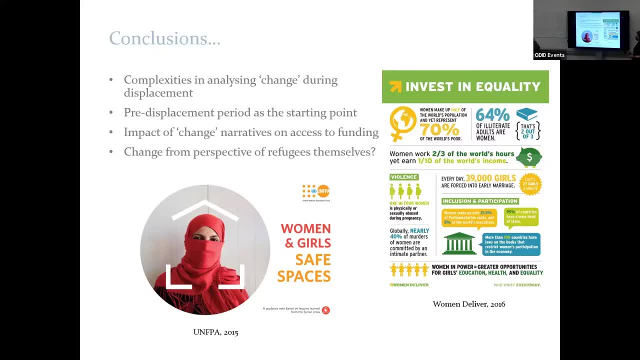 sort of how to place the more disturbing stories that fit into the common narratives. So I think a feminist approach would say that we don't flatten out the complexities and the contradictions but we try to give light and space for them, which I think is quite different. 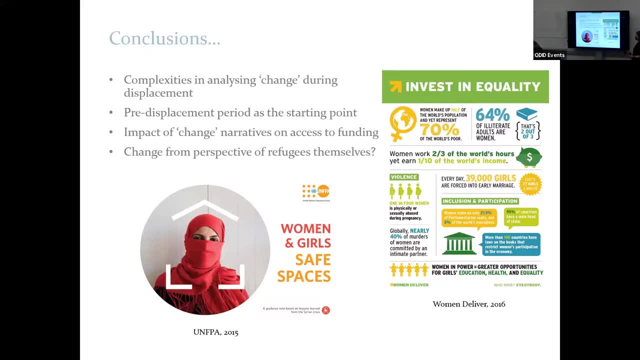 to how humanitarian actors would position it, Because if they were analysing the data- and I know because I did this when I worked for them- you would just choose the most dramatic story or the most compelling narrative that shows what we can do or how we can transform their lives. 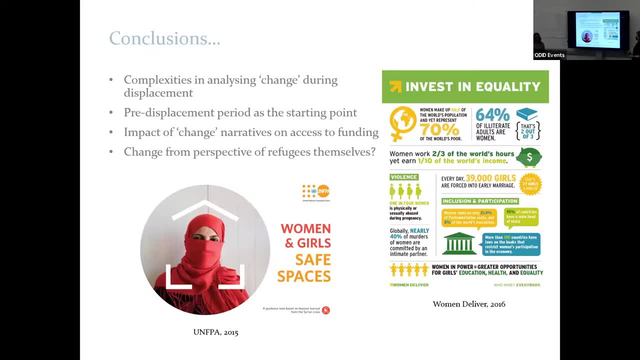 I think definitely. in my research I came across stories, for example, of domestic violence, that really reinforced these narratives. But then for me. so I'm writing a paper at the moment trying to sort of talk about these marital relationships, but it means contextualising them. 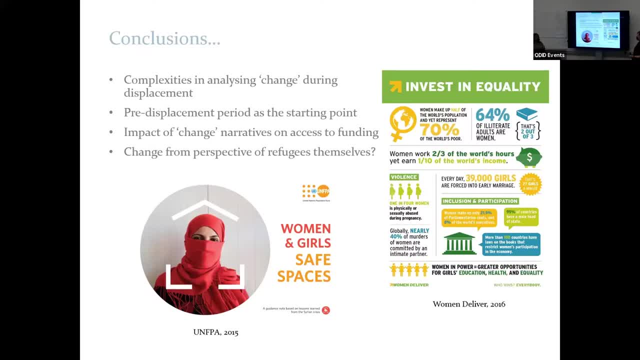 alongside the examples of the positive relationships that other women have, So that it's not that I just sort of pick out the worst stories and put them all in a nice little package and say, look, here is this terrible situation, But it's bringing nuance. 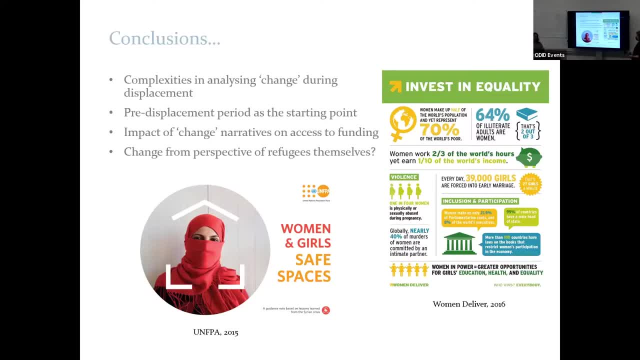 and trying to draw all the different perspectives in And also, I think, not being afraid of not having a tidy narrative. I think people increasingly wanting you to say: well, can you just say what's the one thing that you found? Can you just summarise one takeaway message? 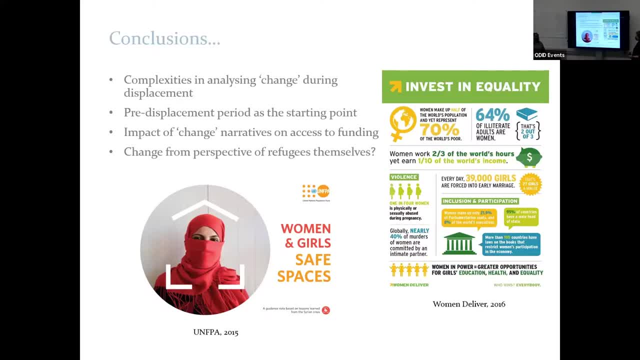 And so then when you say, oh well, it's really complex And there are cases of both positive and negative People aren't satisfied with that because they want something really quick and grabby and snappy, And so I think, trying to disrupt that as much as possible, 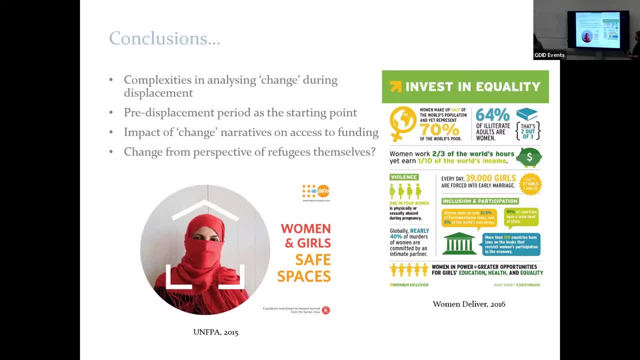 which a lot of feminist writers talk about being happy with living with those contradictions and that uncertainty and where the data doesn't make sense, And actually I've shown both sides of the argument in my paper And so I think that's where that comes in. 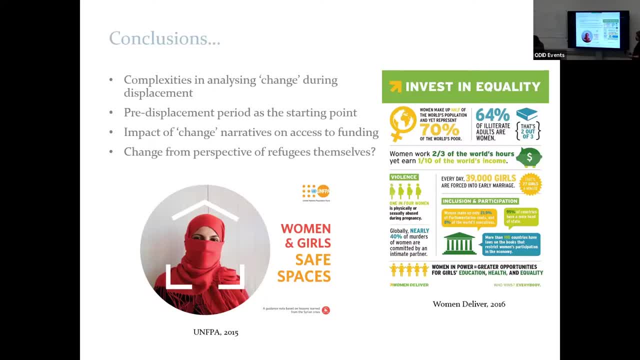 But great question, Yeah. The second question about- I guess really about- patriarchal forces across the world and not just in the countries that we're trying to have. I think that's a really big issue. I think in recent years it seems like there's more appetite towards recognising 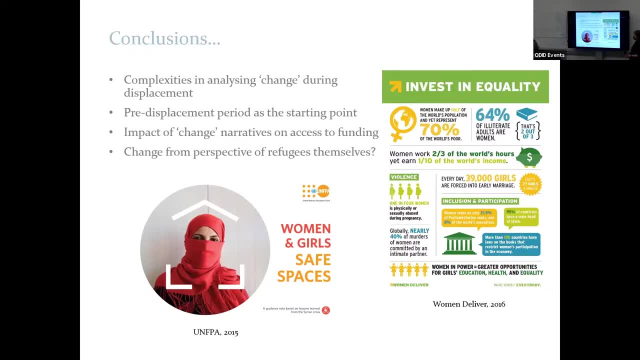 the role of patriarchy and the role of feminist oppression, especially because of the need to use the movement. So it feels like those narratives are coming a lot more to the surface when you hear these stories of women's violence, which is the situation in this order contest. 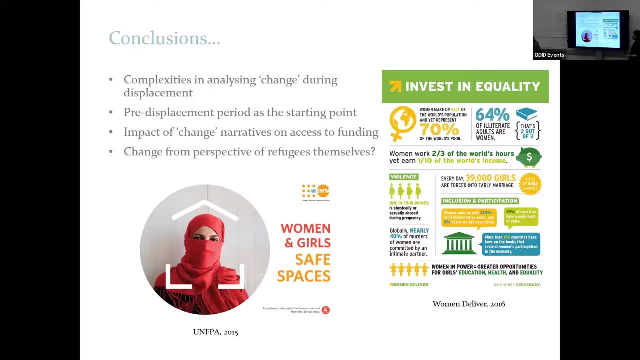 of patriarchy and women's ordination, So it feels like those are coming slightly more to light. But it is true that we are quicker to point out the role of culture, the role of tradition, the gender norms in other settings than we are in a setting like in UK, for example. 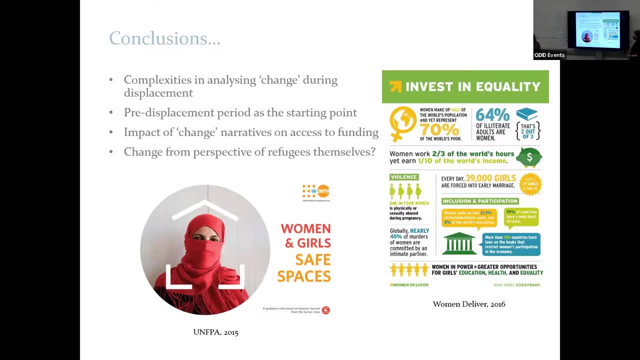 I think that's also part of the critique at the Department of Scholars, where women are saying: why is it always about trying to go over there to help them with their issue and not the child marriage in the US, which is not really a focus? 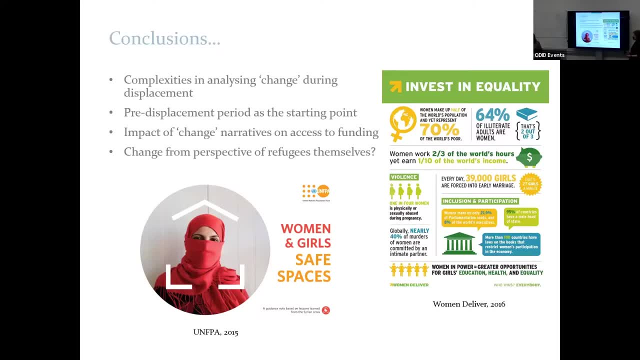 or you don't really hear much about, But there'll be many US organisations who will be doing activities in Sierra Leone and Somalia to end child marriage, And so there are those dissonances, but I'm hopeful that it's starting to shift a little bit. 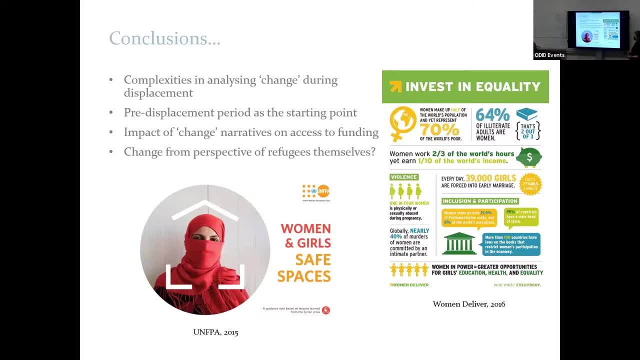 and that I think there's more momentum and I think the women's movement, the feminist movement, has also grown a lot and changed a lot in its messaging, And so hopefully that those kind of dissonances will become a bit more clear. And then the third question. 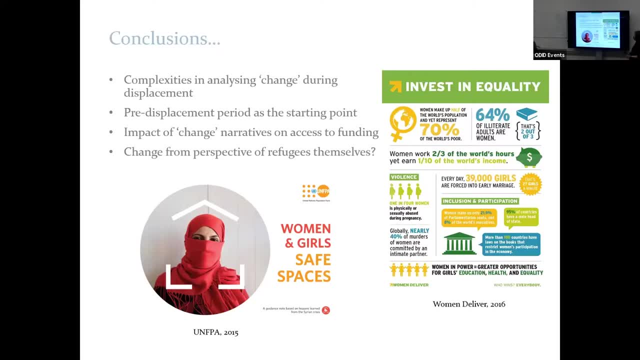 so about relationships between government and the private sector. Yes, I think definitely there are lots of examples. So I'm trying to think of Jordan, where I went, and there were definitely a lot of organisations who wanted to collaborate with humanitarian actors. I do think that might have been one of the earlier slides. 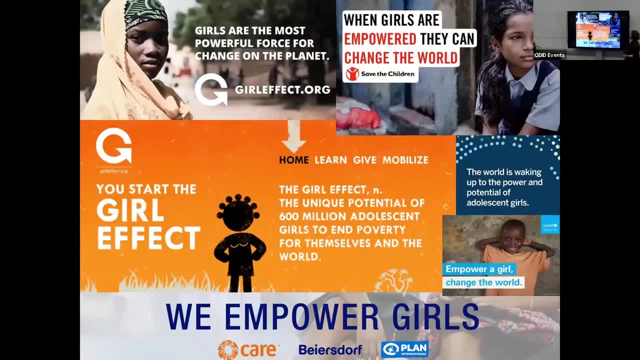 Lots of sometimes smooth grid and sometimes not so good. What is this company, Beersdorf? They are like a skincare company, I think they, and companies like Dove and often will align themselves to sort of women's empowerment and gender equality narratives. 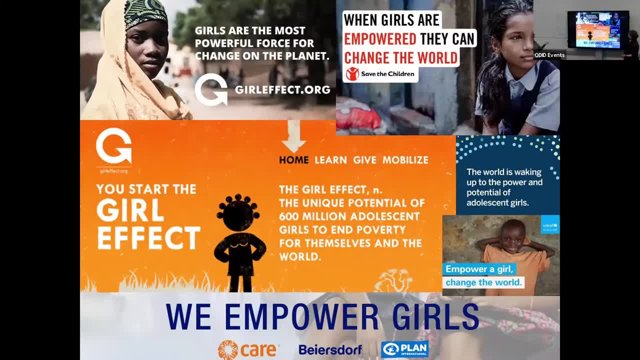 So sometimes it is good because it gives voice and space to that, But then other times it also reinforces certain narratives. So I think there's good and bad sides of government and private sector partnerships, but it's also sometimes ventures feeling like they have to sell a particular perspective. 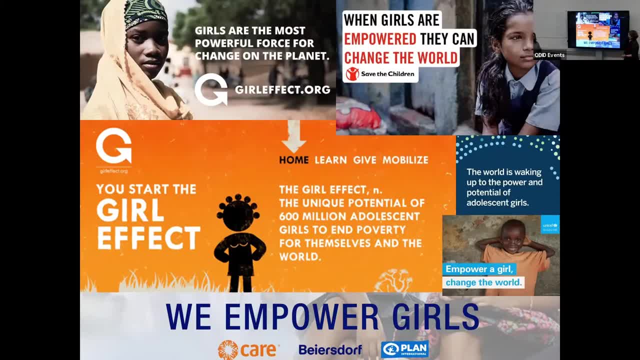 in order to get the attention, or they don't want to downplay the problem because the private sector is not interested, And so having to sort of emphasise how bad the situation is is what makes the funding and the interest as well. We have another few questions. 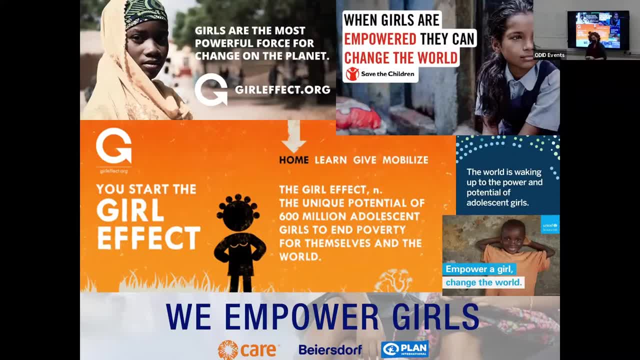 Yes, So you spoke of these narratives that are to make funding possible, Like one that comes to mind, in my mind, is like women's involvement in economic activity, And there are a lot of critiques that are kind of saying that like maybe, women's involvement in economic activity. 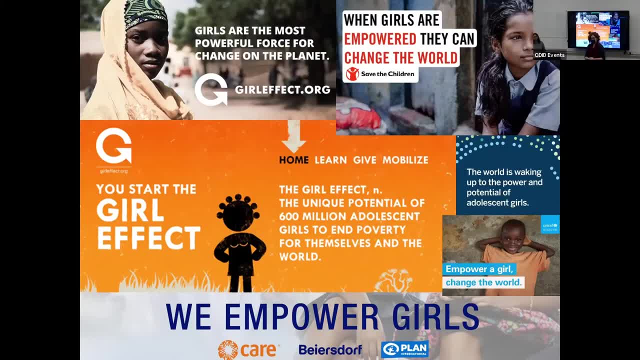 doesn't actually empower them but it's just bringing them into like the capitalist narrative. So I'm curious if we delve into any of that literature and like what the women that you worked with actually expressed to you about like their economic endeavours and aspirations. 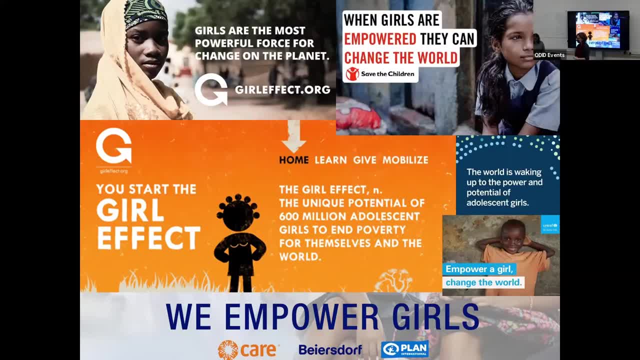 Hi, thank you so much for your talk. That was really interesting. My question is about the term empowerment, which is totally used in international organisations and NGOs And currently, if I'm wrong, my understanding is that they use this term kind of to proclaim themselves as feminists as well. 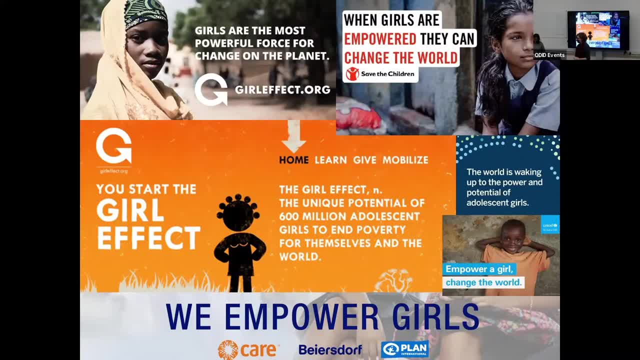 But, as you mentioned, it's also kind of a paradox, because women and men are self-serving at the same time. So how do we, I guess, enter into dialogue with NGOs and doing it more effectively than just like working on women? Yeah, 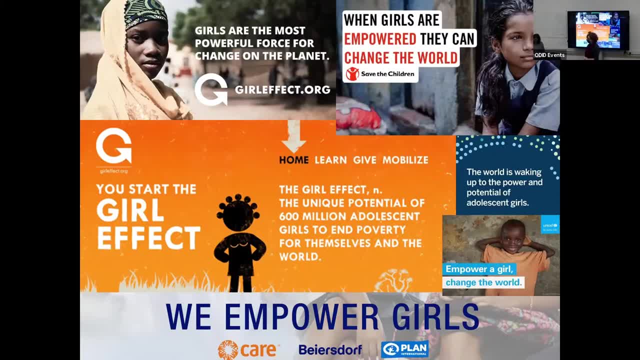 I think you talked about it at the end of your talk. Hi, thank you so much for your talk. I'm Dunar. I'm a member of the teaching staff here at the Refugees for the Culture, And so I wanted to ask you. 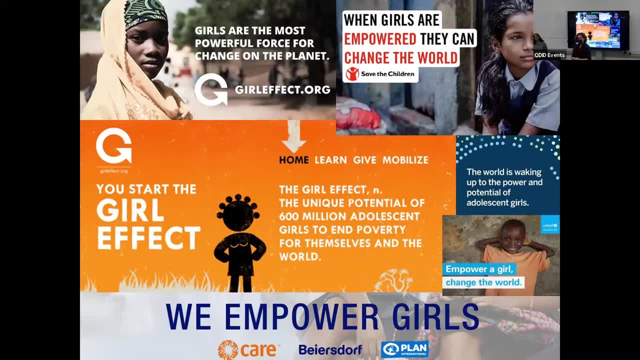 a question about how new gender performance is supposed to create into and a lot of good, critical feminist literature in the region about genderization and how it has also historically undermined more revolutionary anti-capitalist, anti-colonial feminisms in the region. And so now obviously, 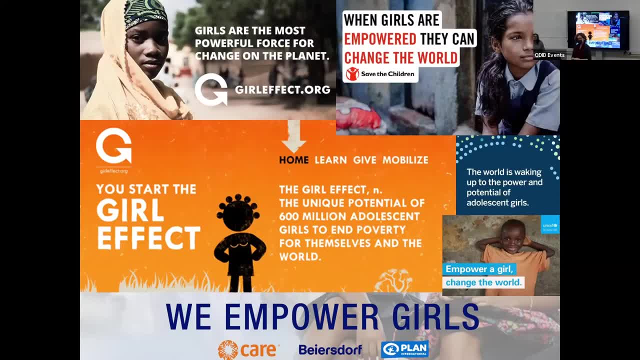 it's been 10 years since the beginning of the Syrian war And, as you described, people have been exposed to all these researchers and humanitarians. And to what extent do you think this dominant tendency among humanitarians to frame experiences along what you described? 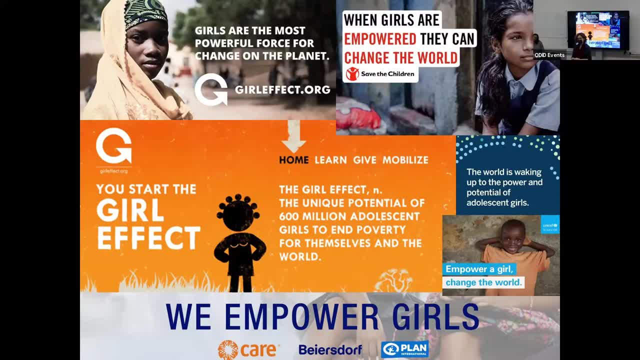 as this neoliberal language of empowerment- and some people have asked questions on this- doesn't only reinforce stereotypes, but also creates new ways in which refugees perform gender. So what I mean is there's incentive, as you described, there's reward for speaking in a certain way. 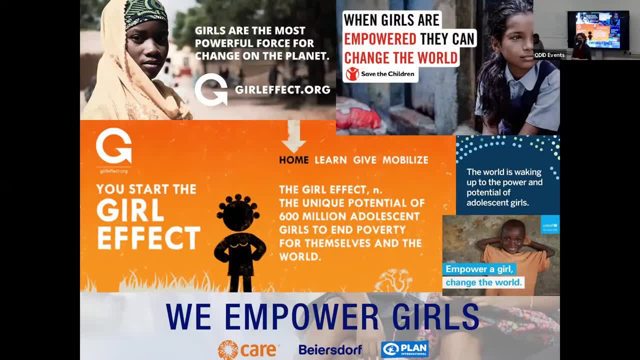 to kind of use this language- that reflects highly Westernized and also very deep politicizing ideas about empowerment and change. So since you've worked in both academia and in the humanitarian sector, I wanted to get any thoughts on how the work of researchers and humanitarians actually sets the tone also. 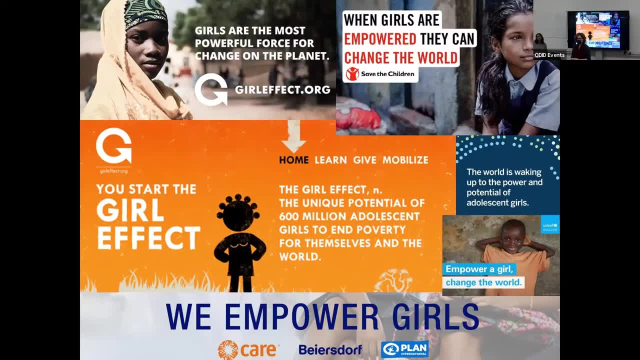 of how refugees speak about their experiences. So any thoughts on that would be appreciated. And I also want to say I really admire your work and I've been assigning it to some of my students since last year. I'll start with that last question. 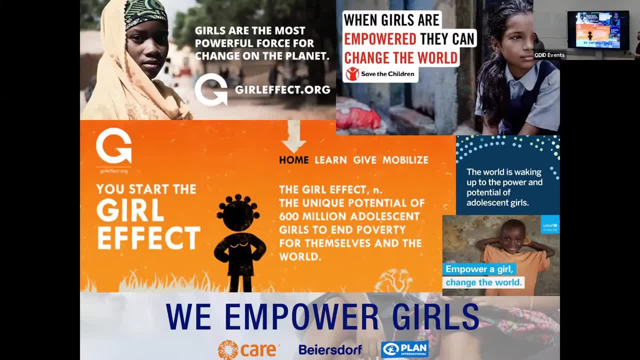 I think it's a really fascinating one to see the way. I think that refugees also understand what people want from them, And I mean the huge amount of researchers just in Jordan alone is astronomical. Like you can't walk down the street without bumping into someone who's doing a PhD. 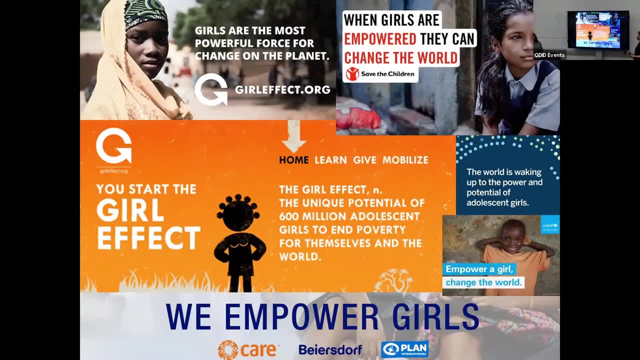 because it's a lot more accessible than a lot of the other countries in the region. It's considered to be safe and the refugees are considered to be much more accessible And so if people have folks there, which I think has created a lot of fatigue on the refugees. 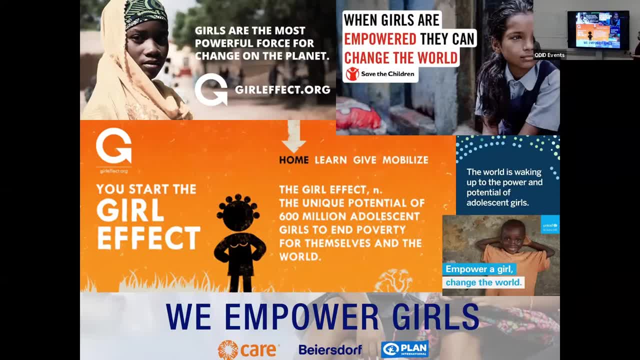 Definitely when I worked. so I worked at the International Rescue Committee, and every time a donor would come, we would trot out the same few refugees who would do their little spiel about being involved in a chemical attack or experiencing violence or experiencing trying to flee. 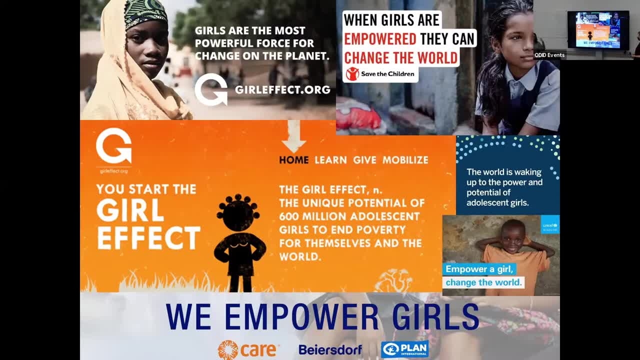 And it was just like they knew what to say. They came into this spiel and then they left, And so there was that constant expectation that you- this is the narrative that we want to hear. I remember in my own PhD research, I was once in a 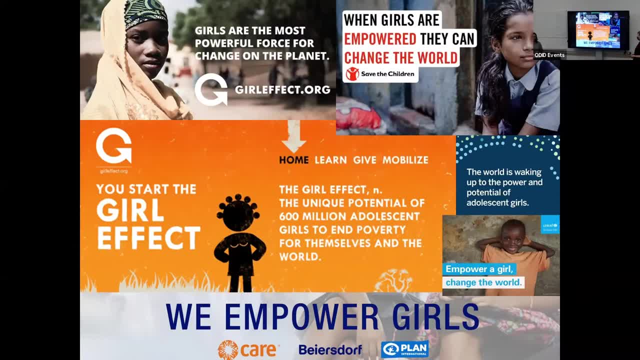 we were doing a focus group discussion and a woman was telling me about her marriage, And then she stopped in the middle and she said: oh, this is not very interesting, You should talk to her. Her story is even worse than mine, And so the assumption is that 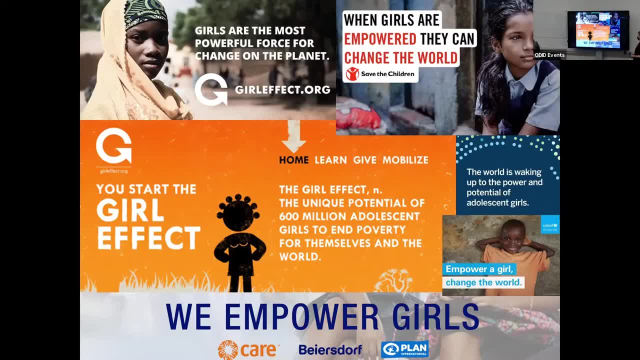 this is what I wanted to hear. I wanted to hear like a really truly terrible story, And that was what they felt: that they had to deliver and had to perform. And I think, yeah, I think definitely. so. who is it? 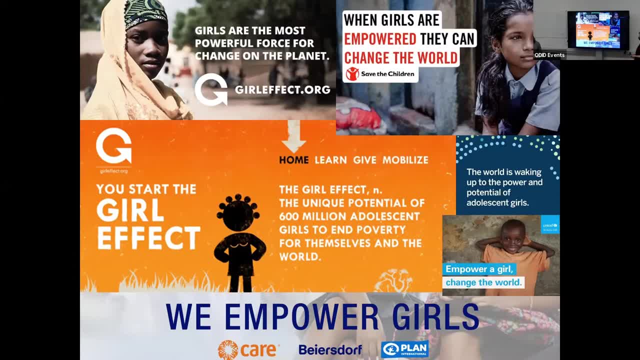 Eleanor Fugui and she did her research that talked about how refugees also sort of perform for the humanitarian active and they acted in the way that was expected for them in order to gain benefits. And I remember at the IRC there were some reports that women were coming to social work. 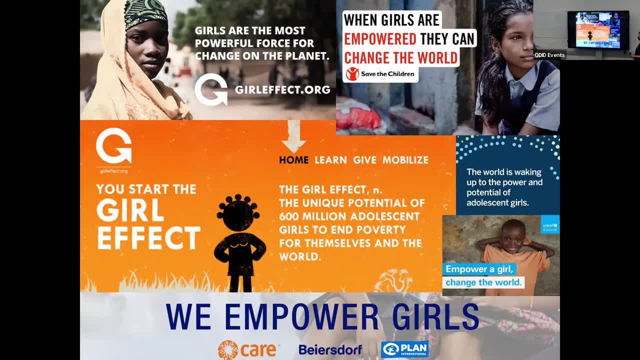 and sort of over-emphasizing their negative experiences, especially over-emphasizing experiences of violence, in order to access cash assistance. Because were they gotten around that to get cash assistance at the IRC, one of the boxes you needed to tick or that would get you somewhere. 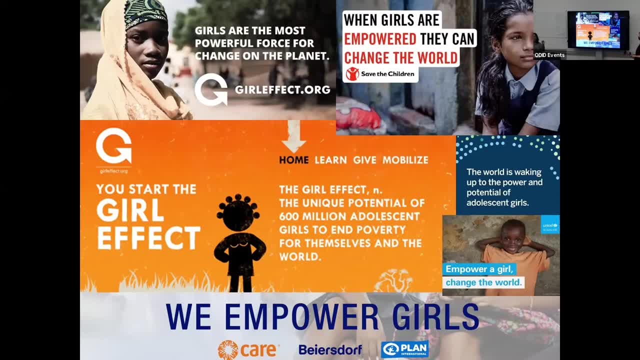 that was huge Free work. and there's all these questions and if you answer yes to a certain number, then you get cash assistance. And so were they gotten around that? if you said you're expert for violence, then you would immediately be fast-tracked to get. 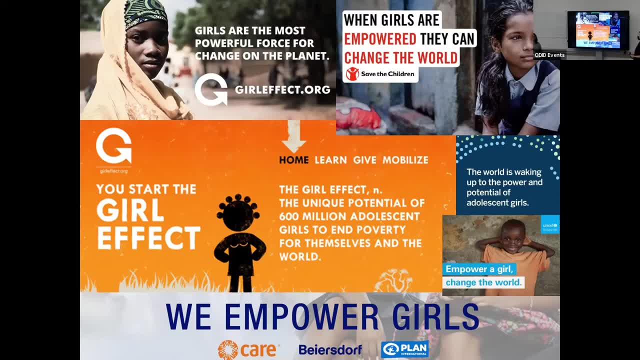 the cash assistance And so refugees, understandably they are living in quite difficult situations. So you do what you can to survive And so I think that is also. I think sometimes there's a bit of judgment when refugees are told they're just trying to take everything. 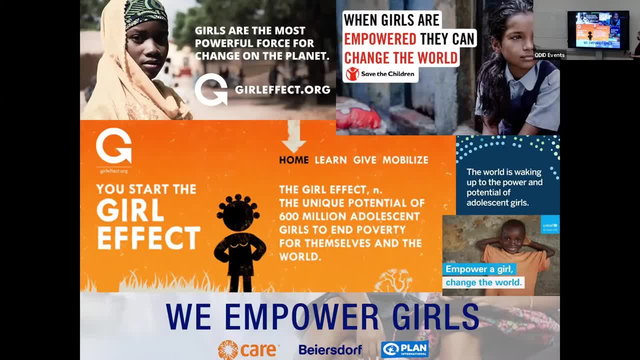 and making up stories. That is what we would probably do if we were in that situation, and in that situation of need, you do whatever it takes to survive. So I think that side of things as well, that performing to survive and then also performing- 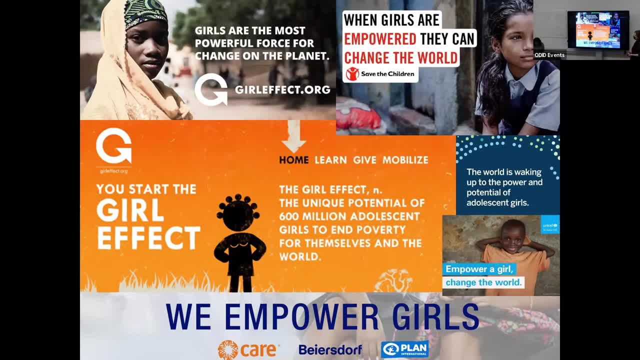 to get different things. And the question, the first question, about neoliberalism. Yes, So I think definitely neoliberalism has crept not just into gender and humanitarian work, but also into feminism, And this maybe ties to the second question as well. 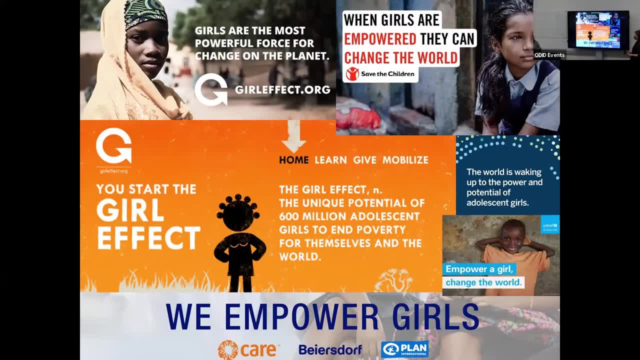 where empowerment used to be about skills and capacity and agency, And there has been a really distinct shift in the last 10, 15 years towards it being economic empowerment, And so that is what it means to be empowered And to truly be empowered. 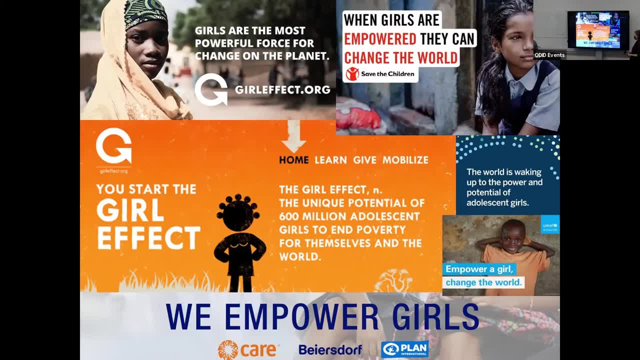 a woman needs to work, she needs to earn money, she needs to have control over her income, which is not necessarily false, but it has really narrowed the scope. And so Andrea Cornwall writes about this. she talks a lot about sort of the way. 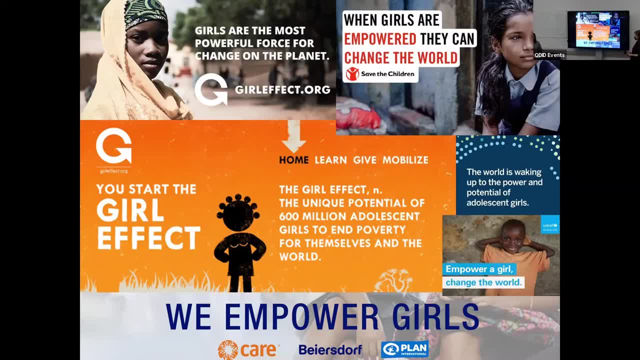 the narrative about empowerment has really shifted and the whole meaning has changed. And I mean now I feel so comfortable to read about empowerment and to write about empowerment, because it's used in such a tokenistic way. It means different things to different people. 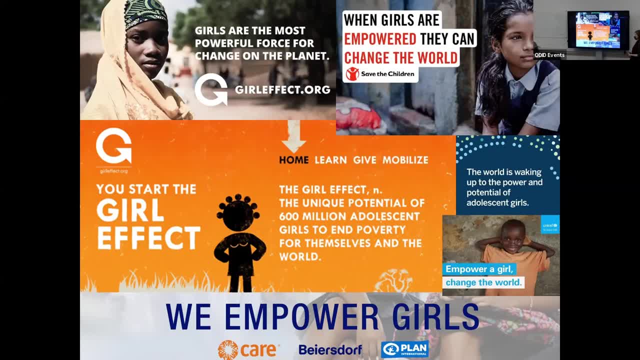 When you say you're empowering a refugee, it immediately conjures up various images and various ideas that may not necessarily be what refugees want or what they need or what they are experiencing or how they would describe it. So I think the neoliberal narrative has really crept into development.